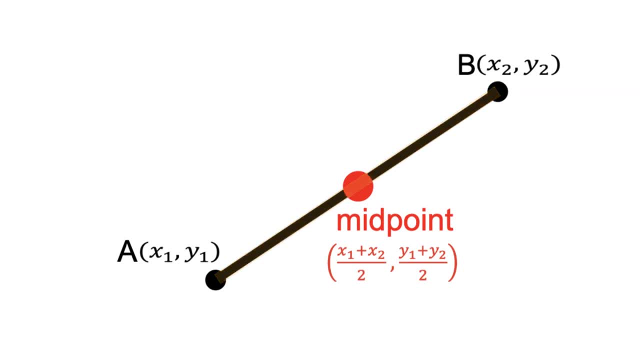 To find the midpoint of line segment a b, we average the x coordinates by adding them and dividing by two, and then we average the y coordinates by adding them and dividing by two, And this will give us the x and y coordinates of the midpoint of the line segment. Let's move on. 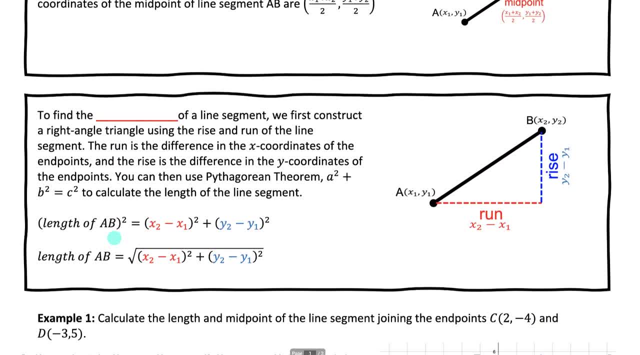 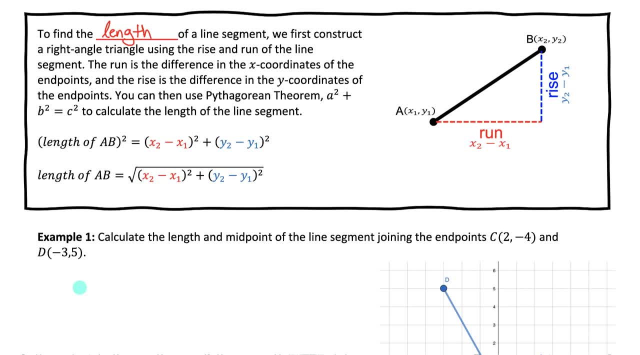 to the length of the line segment formula, and then we'll do some practice questions where we find midpoints and lengths of line segments. So to find the length of a line segment we can use a formula that is generated from our understanding Pythagorean theorem. 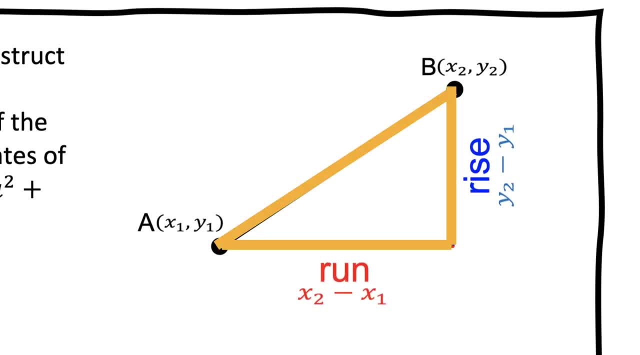 So what we do is we turn the line segment into a right angle triangle by finding its horizontal and vertical components. We call the horizontal component the run and the vertical component the rise. We can calculate the length of the run by finding the difference in the x coordinates. 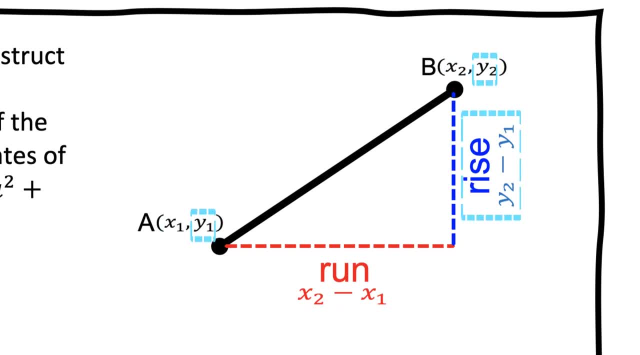 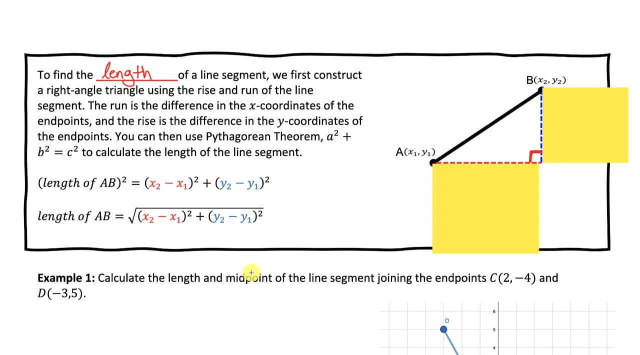 and we can calculate the length of the rise by finding the length of the rise, by finding the difference in the y coordinates. And since this is a right angle triangle, we know that the sum of the squares of the shorter two sides is equal to the square of the longer side, which, in this case, 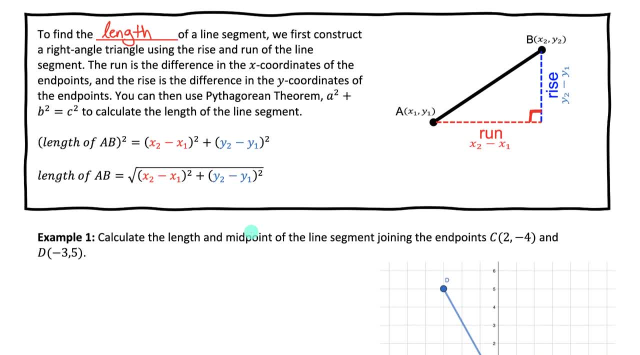 is the line segment that we want the length of. So the length of line segment a- b squared is equal to the difference in the x coordinate squared plus the difference in the y coordinate squared. And if we rearrange to isolate for the length of a- b, we just move the squared to the other side. 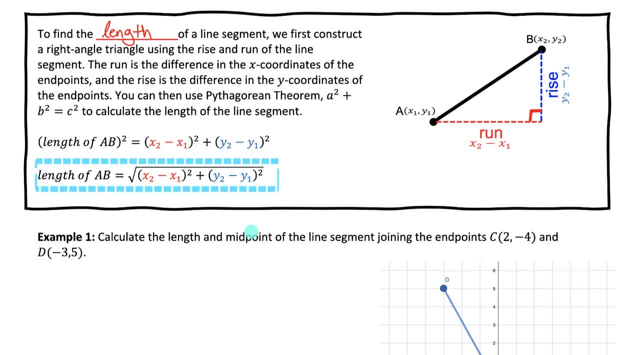 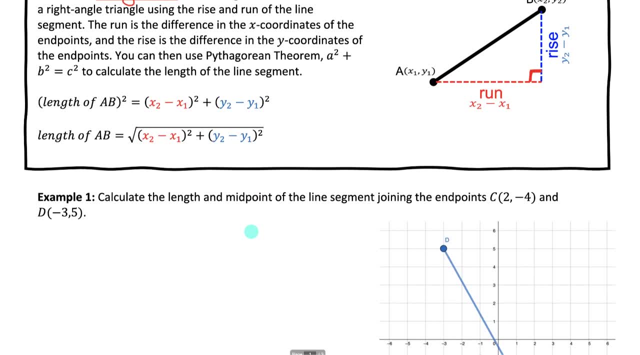 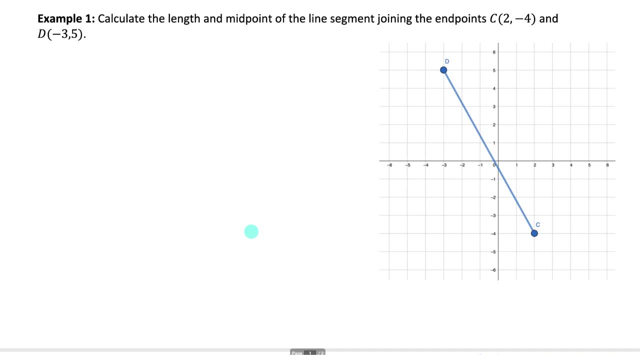 and we end up with the length of a. b equals the square root of the difference in the x coordinate squared plus the difference in the y coordinate squared. Let's practice using those two formulas now. Example one tells us to calculate the length and midpoint of the line segment joining endpoints c and d. 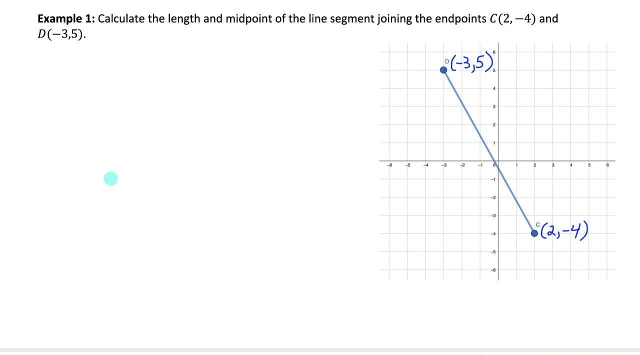 I'm just going to label the points on the diagram and now I'm going to decide which of these two points I want to be my first point and which one I want to be my second point. It doesn't matter which is which, but if we assign each of them to be the first or second point we're going to have. 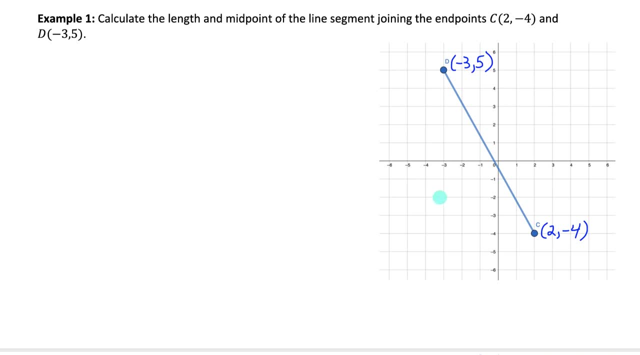 two points that are going to be the first point. So if we assign each of them to be the first point, then we can follow the formula more accurately. I'll let point c be my first point, So I'll call that x1, y1, right, Each point has an x and y coordinate, and since that's my first point, 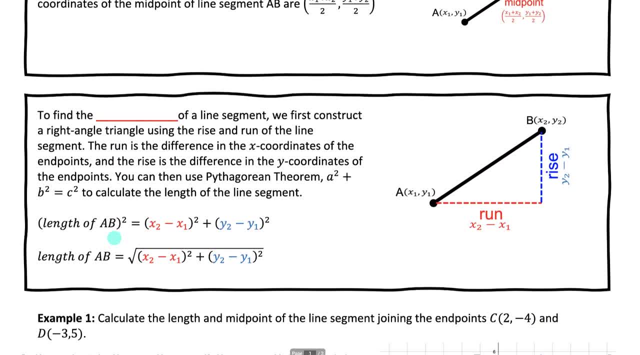 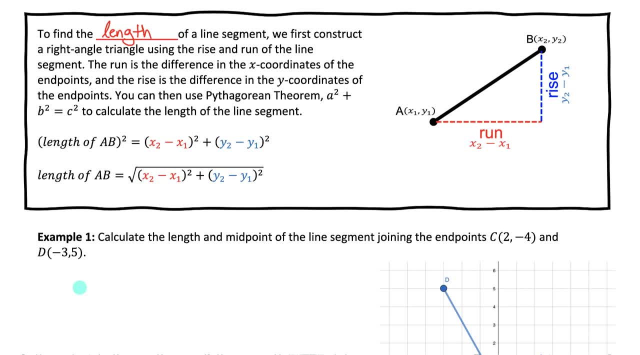 to the length of the line segment formula, and then we'll do some practice questions where we find midpoints and lengths of line segments. So to find the length of a line segment we can use a formula that is generated from our understanding Pythagorean theorem. 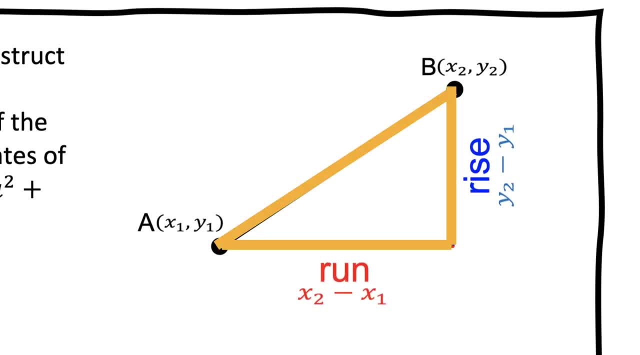 So what we do is we turn the line segment into a right angle triangle by finding its horizontal and vertical components. We call the horizontal component the run and the vertical component the rise. We can calculate the length of the run by finding the difference in the x coordinates. 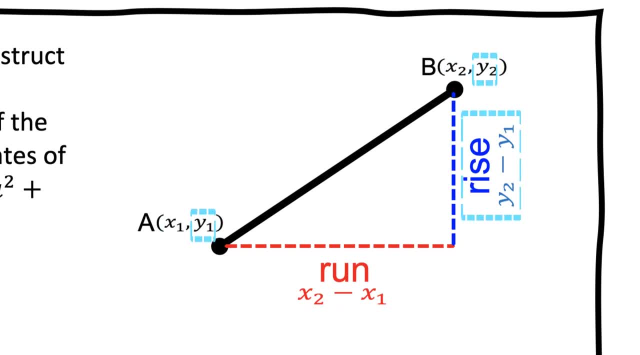 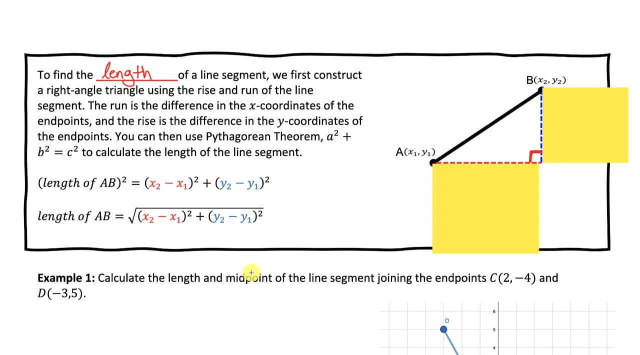 and we can calculate the length of the rise by finding the length of the rise, by finding the difference in the y coordinates. And since this is a right angle triangle, we know that the sum of the squares of the shorter two sides is equal to the square of the longer side, which, in this case, 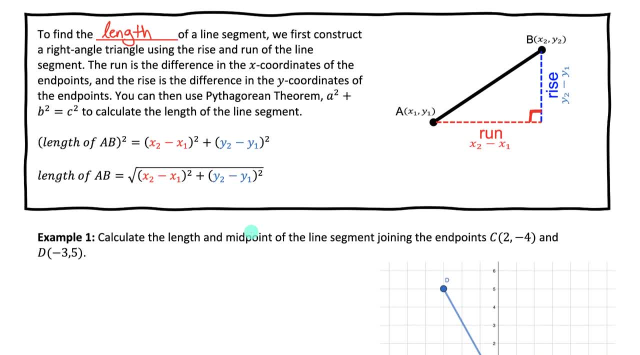 is the line segment that we want the length of. So the length of line segment a- b squared is equal to the difference in the x coordinate squared plus the difference in the y coordinate squared. And if we rearrange to isolate for the length of a- b, we just move the squared to the other side. 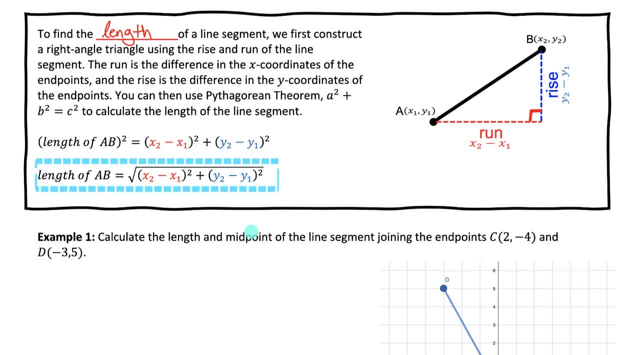 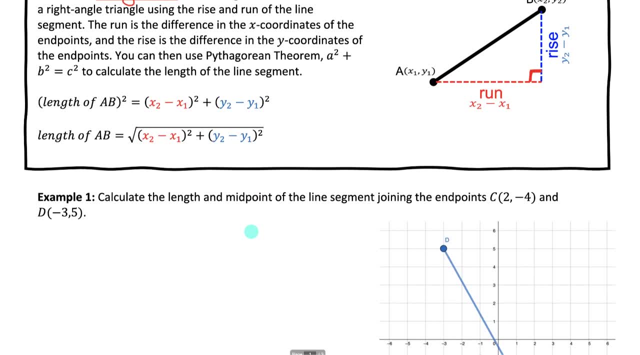 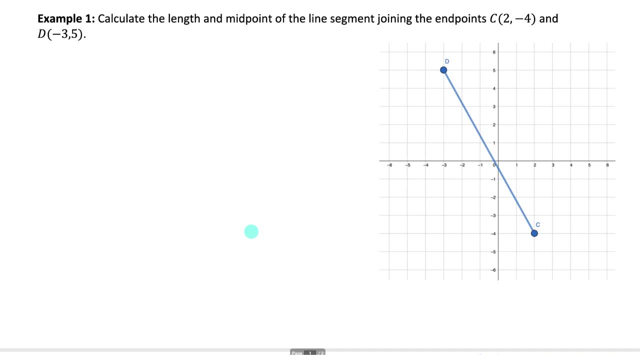 and we end up with the length of a. b equals the square root of the difference in the x coordinate squared plus the difference in the y coordinate squared. Let's practice using those two formulas now. Example one tells us to calculate the length and midpoint of the line segment joining endpoints c and d. 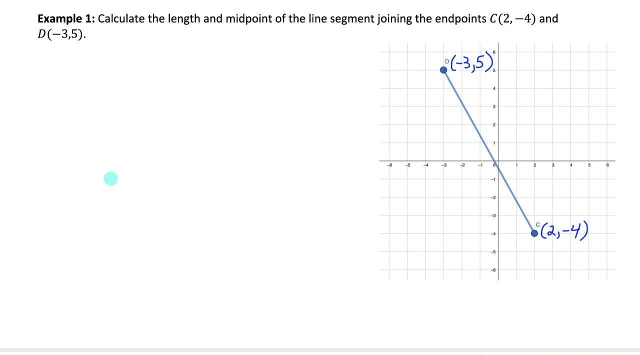 I'm just going to label the points on the diagram and now I'm going to decide which of these two points I want to be my first point and which one I want to be my second point. It doesn't matter which is which, but if we assign each of them to be the first or second point we're going to have. 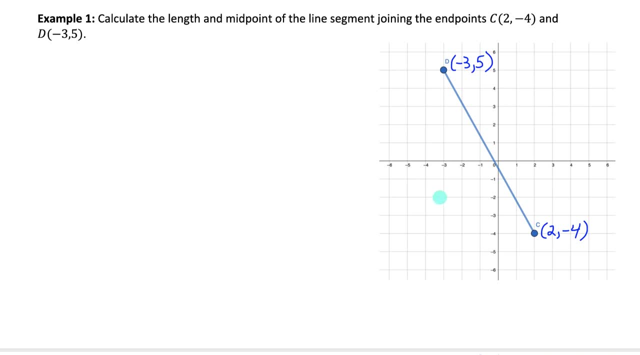 two points that are going to be the first point. So if we assign each of them to be the first point, then we can follow the formula more accurately. I'll let point c be my first point, So I'll call that x1, y1, right, Each point has an x and y coordinate, and since that's my first point, 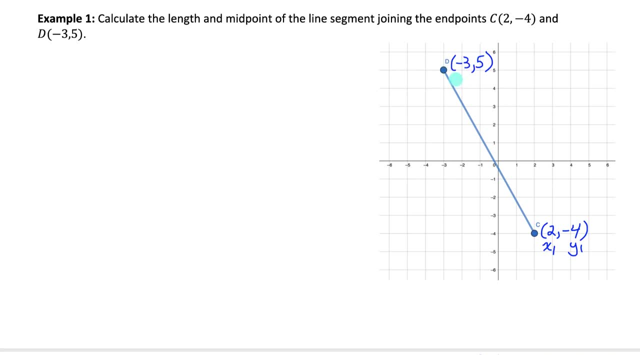 I'll call that x1, y1.. And my second point is point d, so I'll call those coordinates x2 and y2.. Now, if I'm going to find the midpoint of line segment c d, I'll short form that by saying the: 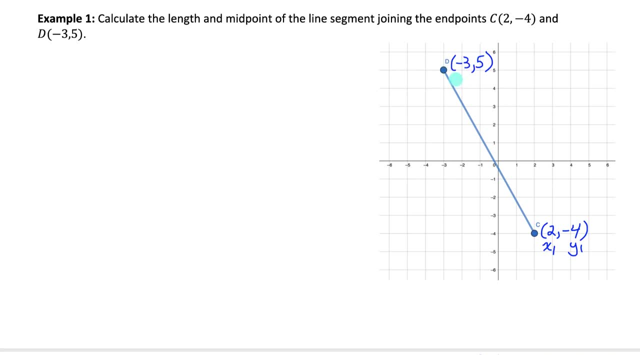 I'll call that x1, y1.. And my second point is point d, so I'll call those coordinates x2 and y2.. Now, if I'm going to find the midpoint of line segment c d, I'll short form that by saying the: 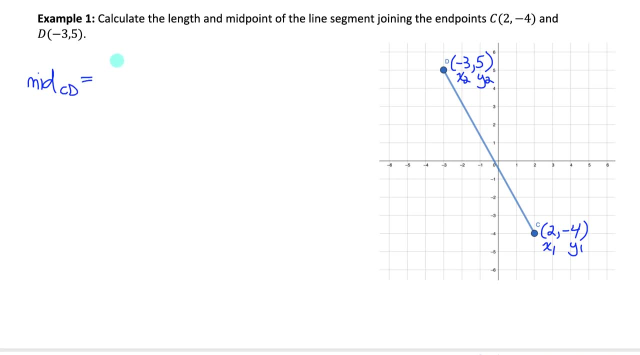 mid of line segment c, d equals. I can find the coordinates of the midpoint by following the formula which tells me to find the average of the x coordinates, and I do that by adding them and dividing by 2.. So I'll do x1. 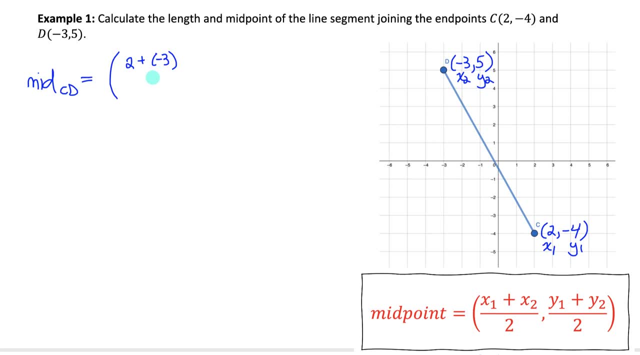 plus x2, divided by 2.. That'll get me the x coordinate of the midpoint, and I can find the y coordinate of the midpoint by adding the y coordinates and dividing by 2.. So I'll do y1,, which is negative, 4,, plus y2, which is 5, divide that by 2.. 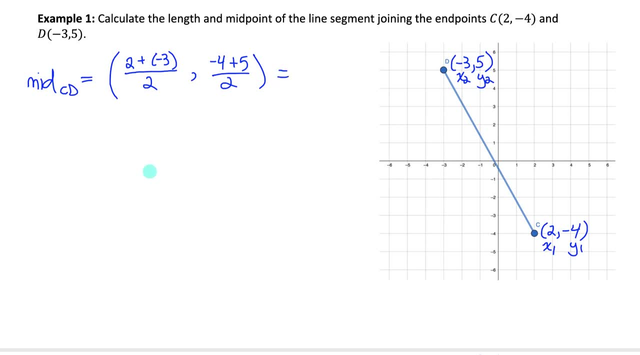 And now I'll simplify the x and y coordinates. If I look at the x coordinate of the midpoint, 2 plus negative 3 is negative 1.. So my x coordinate is negative 1 over 2.. And my y coordinate, negative 4 plus 5 is 1, and that's over 2.. So my midpoint is at negative 1 half, 1 half. 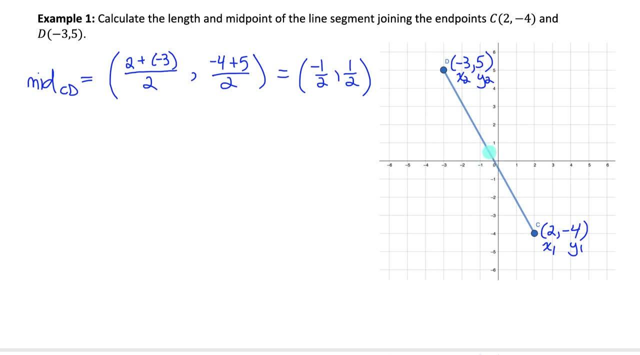 If I were to plot that point, if I were to move to negative 1 half, 1 half, I would notice that that point is on the line segment and that looks like that's right in the middle of the line segment. That's my midpoint. It's at negative 1 half, 1 half. 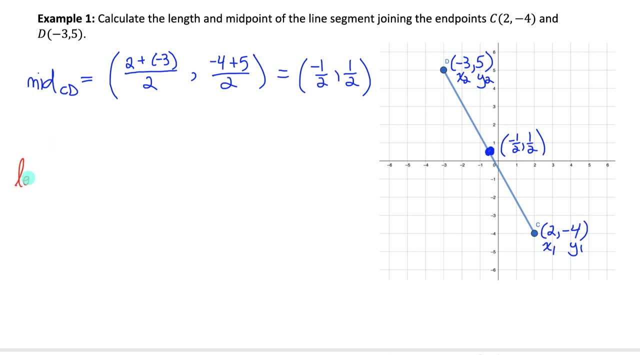 Now I'll find the length of line segment CD. So I'll say the length of CD equals, and if I follow the formula for length of the line segment, I need to find the difference in the x coordinates. So I'll do x2 minus x1, that's negative 3 minus 2 squared plus the. 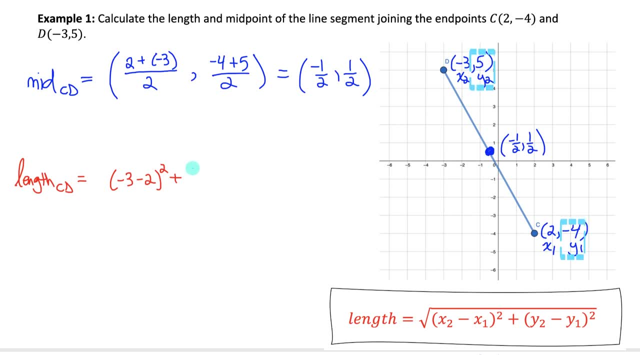 difference in the y coordinates. So I'll do y2 minus y1,, which would be 5 minus negative 4, squared, And that all needs to be square rooted. And let me actually simplify: under the square root here, Negative 3 minus 2 is negative 5, and 5 minus negative 4 is 9.. Now 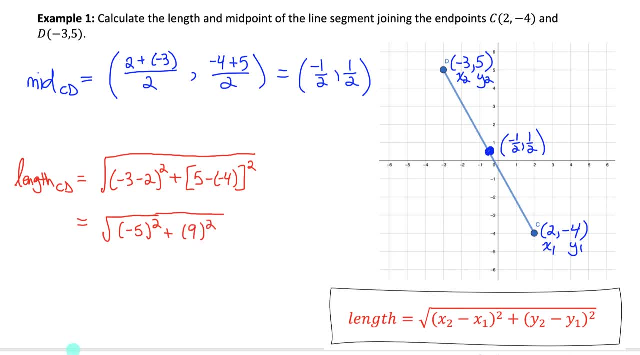 I won't always show this step, but I think it's important for me to show it here to help you understand how this formula is actually going to tell us the length of the line segment. The absolute value of the difference in the x's is 5, and notice. 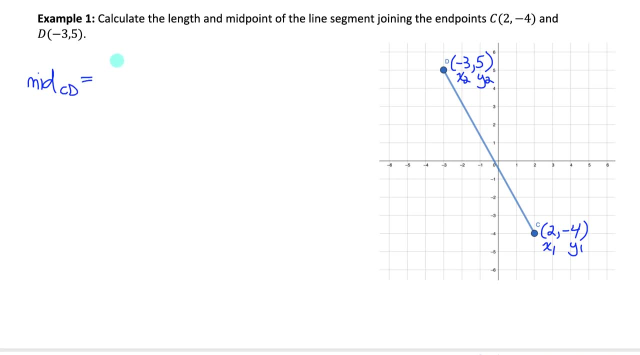 mid of line segment c, d equals. I can find the coordinates of the midpoint by following the formula which tells me to find the average of the x coordinates, and I do that by adding them and dividing by 2.. So I'll do x1. 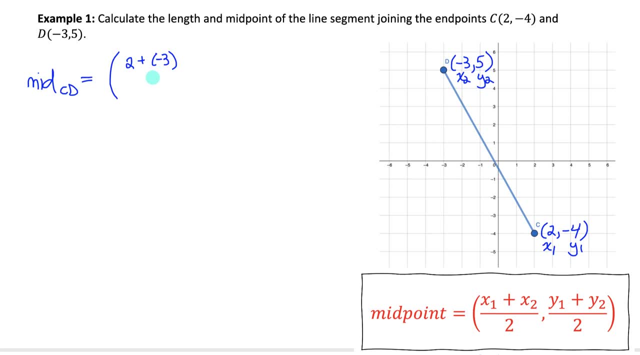 plus x2, divided by 2.. That'll get me the x coordinate of the midpoint, and I can find the y coordinate of the midpoint by adding the y coordinates and dividing by 2.. So I'll do y1,, which is negative, 4,, plus y2, which is 5, divide that by 2.. 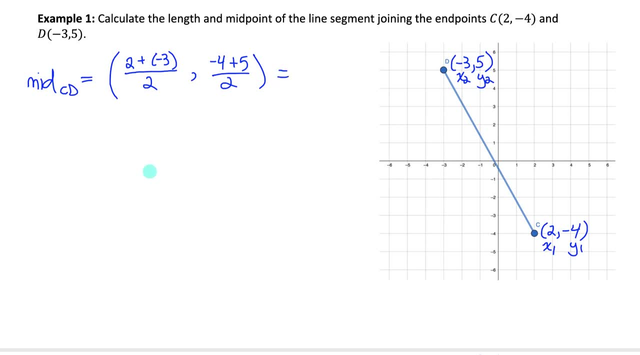 And now I'll simplify the x and y coordinates. If I look at the x coordinate of the midpoint, 2 plus negative 3 is negative 1.. So my x coordinate is negative 1 over 2.. And my y coordinate, negative 4 plus 5 is 1, and that's over 2.. So my midpoint is at negative 1 half, 1 half. 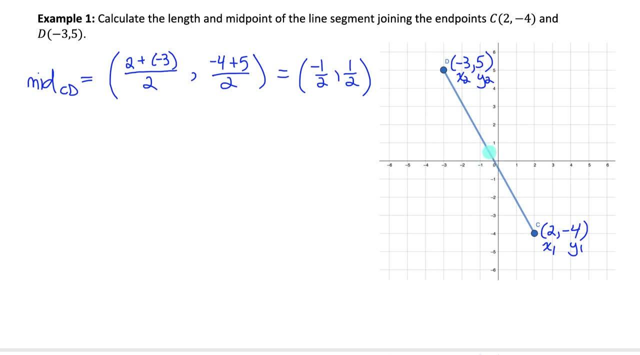 If I were to plot that point, if I were to move to negative 1 half, 1 half, I would notice that that point is on the line segment and that looks like that's right in the middle of the line segment. That's my midpoint. It's at negative 1 half, 1 half. 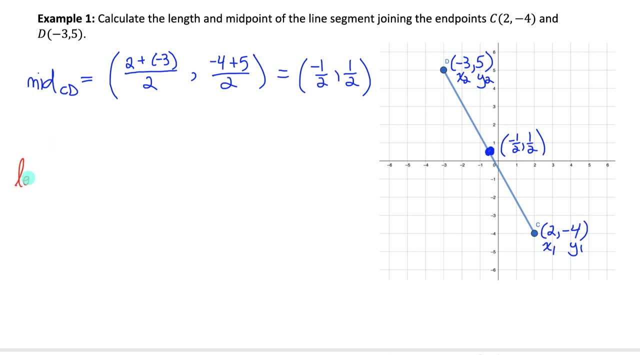 Now I'll find the length of line segment CD. So I'll say the length of CD equals, and if I follow the formula for length of the line segment, I need to find the difference in the x coordinates. So I'll do x2 minus x1, that's negative 3 minus 2 squared plus the. 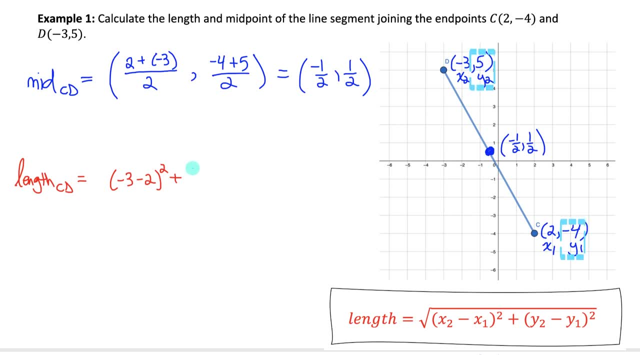 difference in the y coordinates. So I'll do y2 minus y1,, which would be 5 minus negative 4, squared, And that all needs to be square rooted. And let me actually simplify: under the square root here, Negative 3 minus 2 is negative 5, and 5 minus negative 4 is 9.. Now 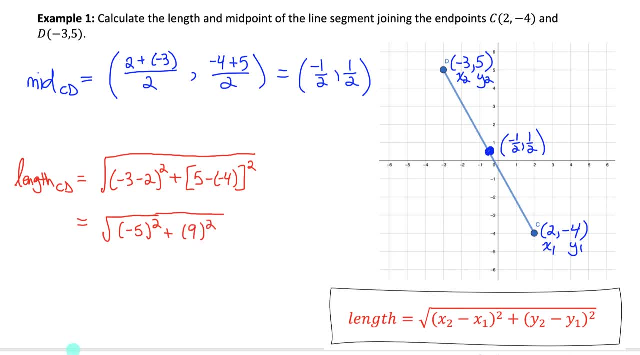 I won't always show this step, but I think it's important for me to show it here to help you understand how this formula is actually going to tell us the length of the line segment. The absolute value of the difference in the x's is 5, and notice. 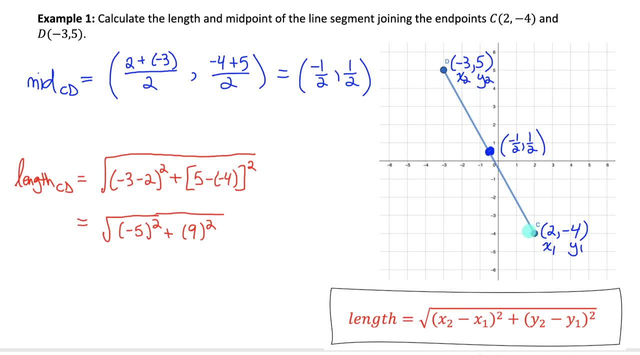 if I were to make this into a right triangle by drawing its horizontal and vertical components. the length of the horizontal component is 5 units and the length of the vertical component is 9 units, And what we know, based on Pythagorean theorem, is that the sum of the squares of 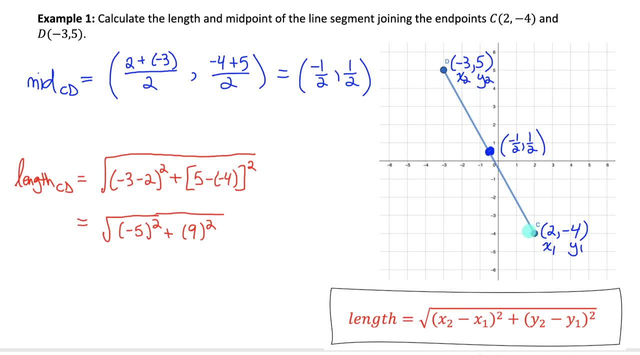 if I were to make this into a right triangle by drawing its horizontal and vertical components. the length of the horizontal component is 5 units and the length of the vertical component is 9 units, And what we know, based on Pythagorean theorem, is that the sum of the squares of 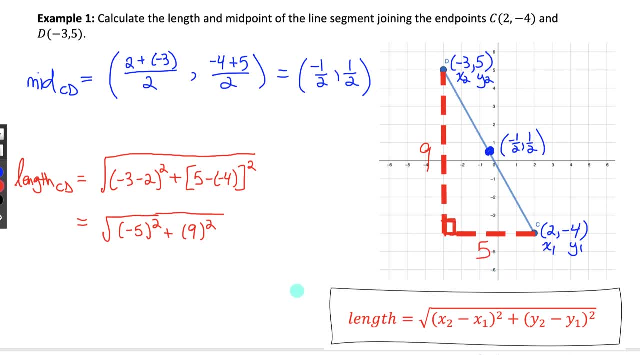 the shorter two sides- 5 and 9, should be equal to the square of the longer side, the line segment CD, which is what we're trying to find. So that's where this formula comes from. Now, I know I said the length of this is. 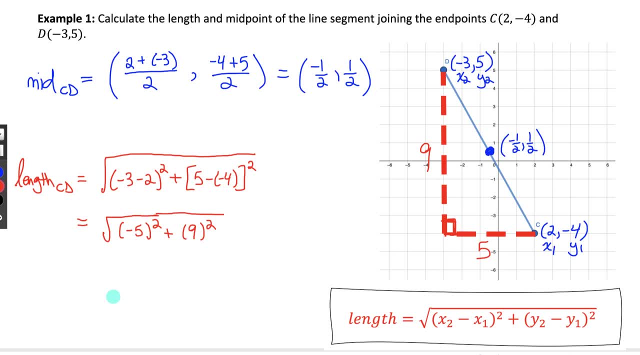 5, and here I see a negative 5,. but when we square it's going to work out to the same thing. Just the absolute value of the difference tells us the length of the lines, and that's why Pythagorean theorem allows us to find the length of the line segment. But if we 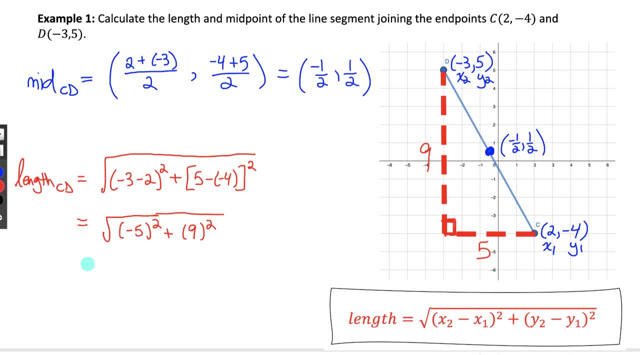 follow the formula, it'll all work out the way we want it to. So, if I simplify, under the square root I have negative 5 squared, which is 25, plus 9 squared, which is 81. So 25 plus 81 is 106, so I have the square root of 106.. That's the exact length. 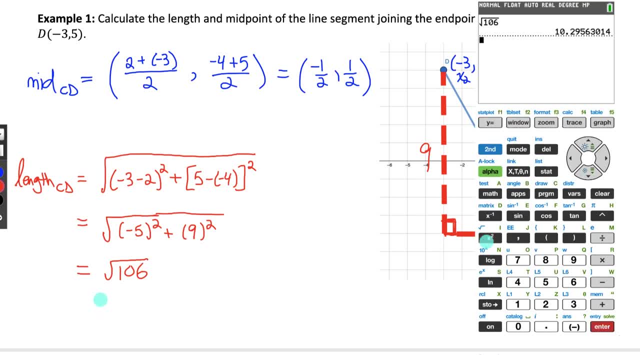 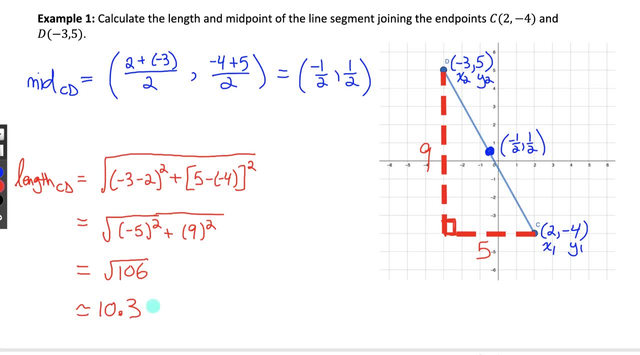 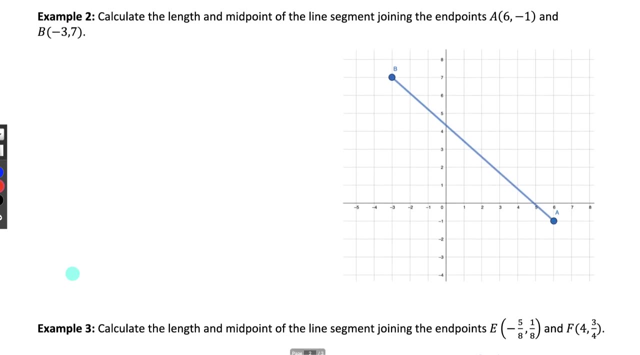 If I want the approximate length, I can evaluate that on my calculator and I would get a value of about 10.3.. And I don't know what units I'm in, so I could just write 10.3 units. Let's try another example, Example 2.. We'll calculate the length and midpoint of the line. 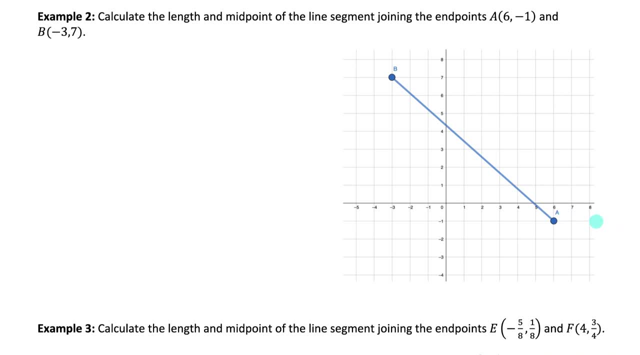 segment joining A and B. So once again, let me label the points on the graph and I'll choose point A to be my first point, So that's my x1, y1.. And point B to be my second point, That's my x2, y2.. If I'm going to find the midpoint, 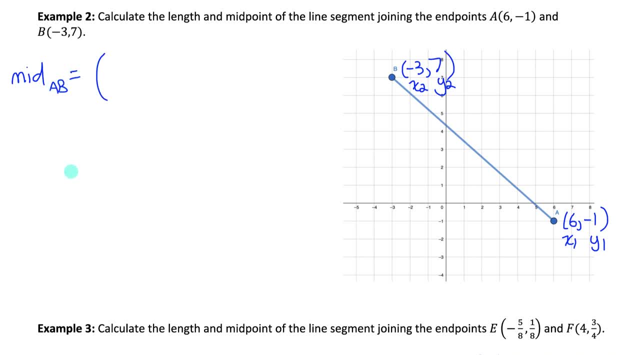 of line segment A B, I need to average the x coordinates. If I follow the formula, it tells me to do x1 plus x2, and then divide by 2.. So 6 plus negative 3 over 2.. And then 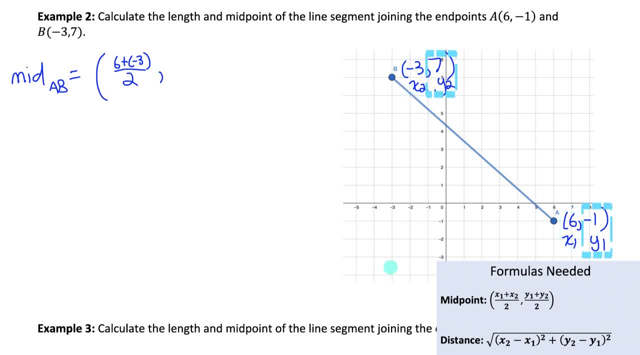 to get the y coordinate of the midpoint, I need to average the y coordinates of my endpoints. So y1 plus y2 is negative 1 plus 7.. And then I need to divide that by 2 to find the average. If I simplify this, 6 plus negative 3 is 3, so I have 3 over 2, which I suppose I could. 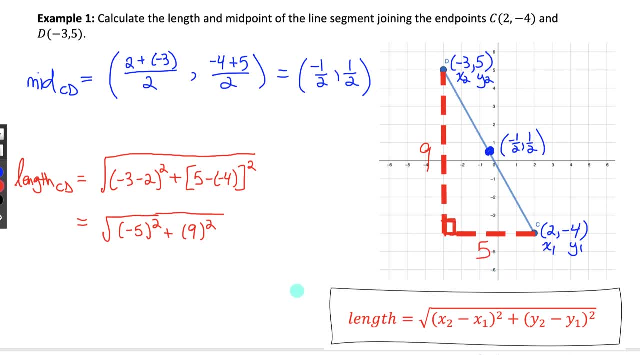 the shorter two sides- 5 and 9, should be equal to the square of the longer side, the line segment CD, which is what we're trying to find. So that's where this formula comes from. Now, I know I said the length of this is. 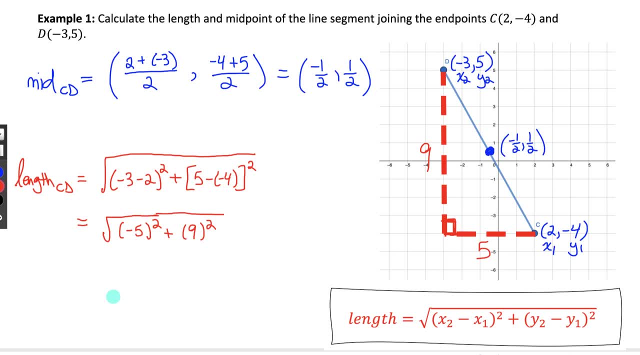 5, and here I see a negative 5,. but when we square it's going to work out to the same thing. Just the absolute value of the difference tells us the length of the lines, and that's why Pythagorean theorem allows us to find the length of the line segment. But if we 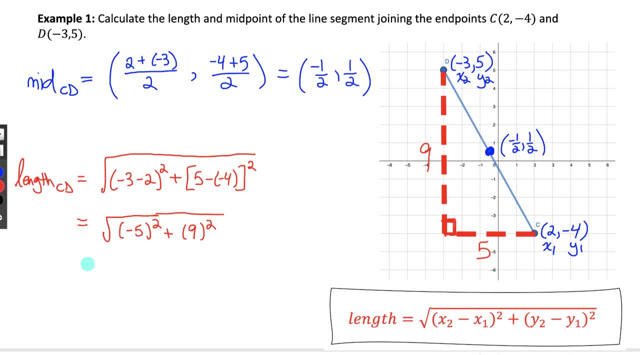 follow the formula, it'll all work out the way we want it to. So, if I simplify, under the square root I have negative 5 squared, which is 25, plus 9 squared, which is 81. So 25 plus 81 is 106, so I have the square root of 106.. That's the exact length. 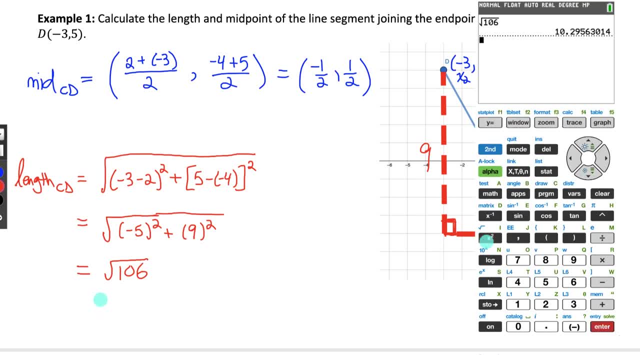 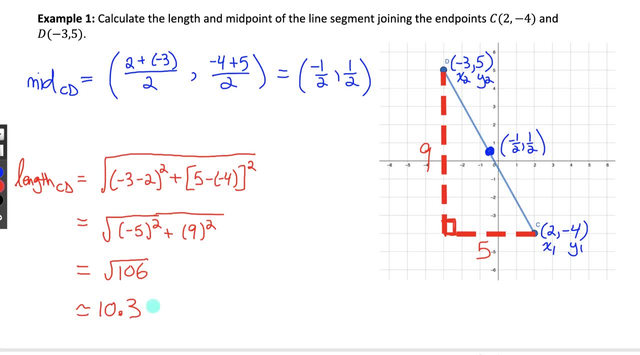 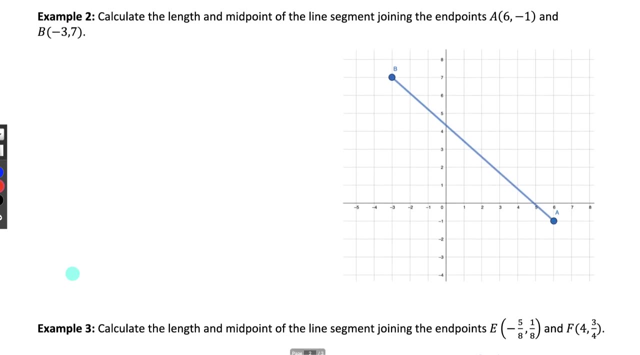 If I want the approximate length, I can evaluate that on my calculator and I would get a value of about 10.3.. And I don't know what units I'm in, so I could just write 10.3 units. Let's try another example, Example 2.. We'll calculate the length and midpoint of the line. 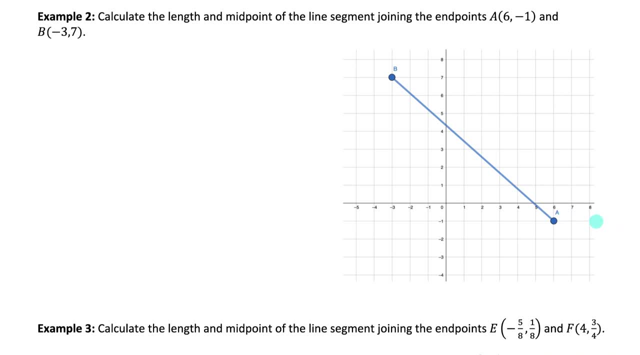 segment joining A and B. So once again, let me label the points on the graph and I'll choose point A to be my first point, So that's my x1, y1.. And point B to be my second point, That's my x2, y2.. If I'm going to find the midpoint, 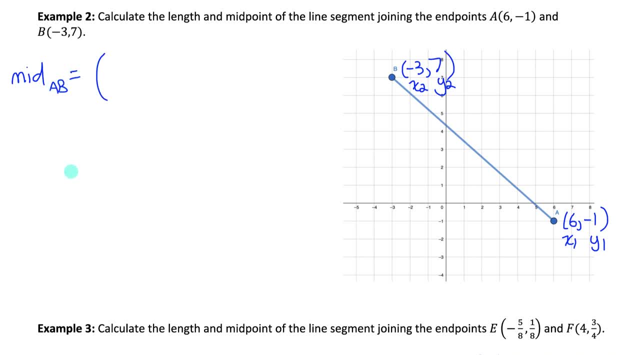 of line segment A B, I need to average the x coordinates. If I follow the formula, it tells me to do x1 plus x2, and then divide by 2.. So 6 plus negative 3 over 2.. And then 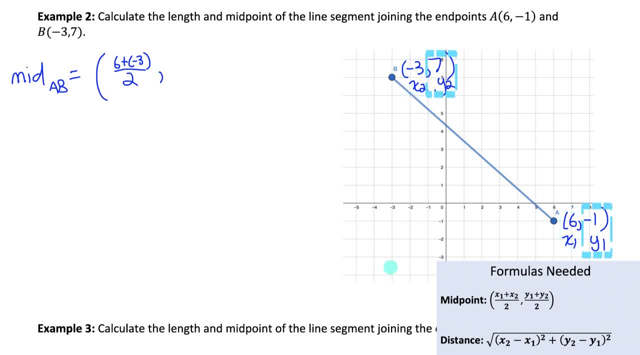 to get the y coordinate of the midpoint, I need to average the y coordinates of my endpoints. So y1 plus y2 is negative 1 plus 7.. And then I need to divide that by 2 to find the average. If I simplify this, 6 plus negative 3 is 3, so I have 3 over 2, which I suppose I could. 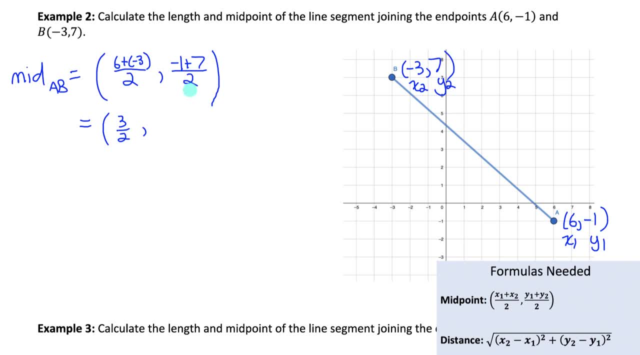 write as 1.5,, but I'll leave it as a fraction, And the y coordinate of the midpoint is negative. 1 plus 7, which is 6, over 2, which 6 divided by 2 is 3.. 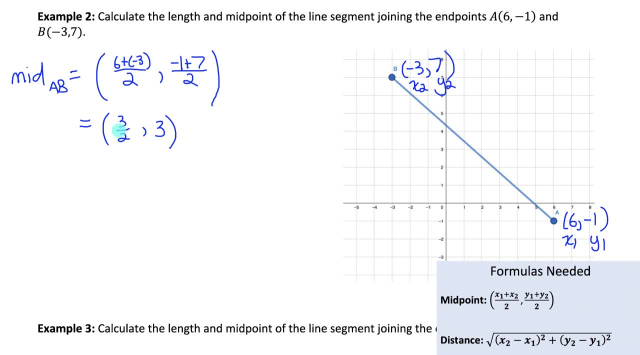 Let's check if that midpoint looks right on our line segment. The point 1.53 is right here. It appears to be on the line and it appears to be right in the middle of the line. So it looks like we have the right midpoint. 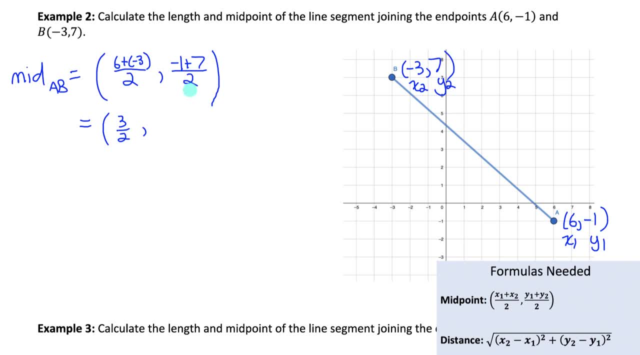 write as 1.5,, but I'll leave it as a fraction, And the y coordinate of the midpoint is negative. 1 plus 7, which is 6, over 2, which 6 divided by 2 is 3.. 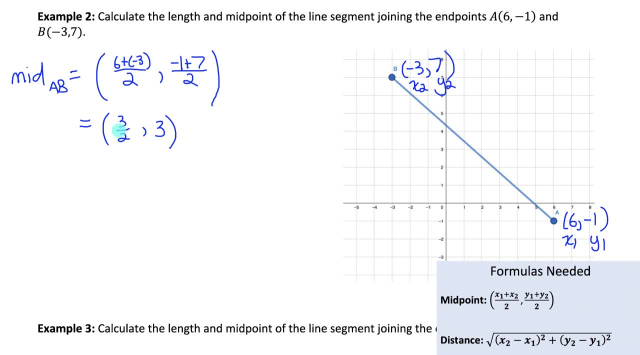 Let's check if that midpoint looks right on our line segment. The point 1.53 is right here. It appears to be on the line and it appears to be right in the middle of the line. So it looks like we have the right midpoint. 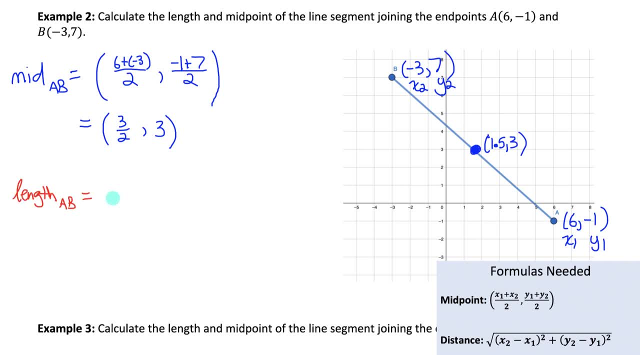 To find the length of line segment AV and to find the length we need to square root the difference in the x's squared plus the difference in the y's squared. So we'll do the difference in the x coordinates and we'll follow what the formula tells us to do. We'll 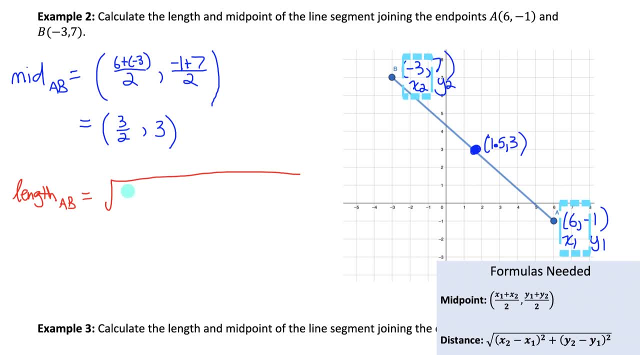 do x2 minus x1, so negative 3 minus 6, squared plus the difference in the y coordinates, And the formula says to do y2 minus y1, so I will do 7 minus negative 1.. I'm gonna do 7 minus 8 squared. If I simplify underneath the square root, I would have negative. 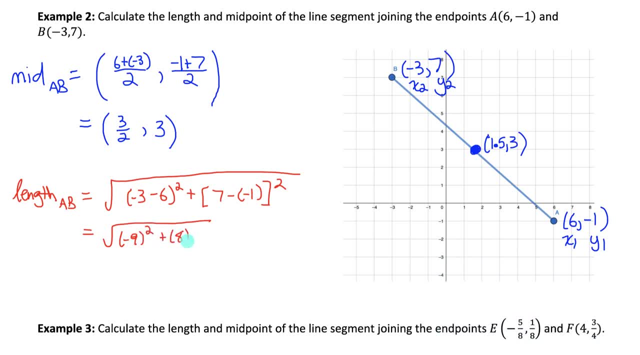 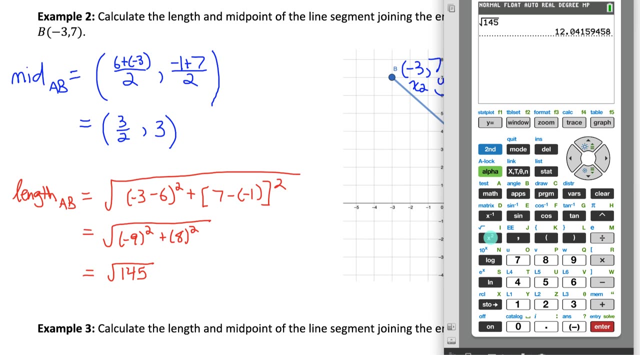 9 squared plus 8 squared. If I collect those terms under the square root, I would have the square root of 145 as my exact answer. If I want an approximate answer, I can type that on my calculator and I get approximately 12.04 units And hopefully you remember why. 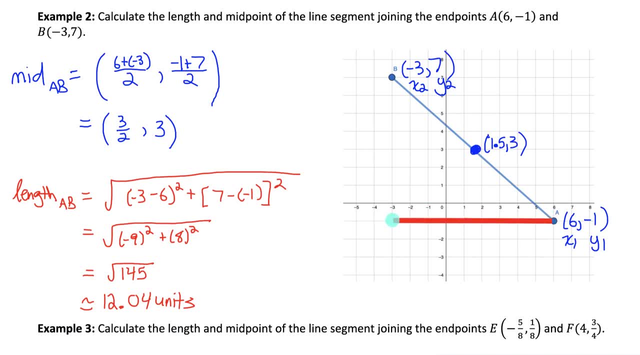 that formula works really. what we did was we used pythagorean theorem. by turning this into a right triangle and by finding the difference in the x coordinates, we found out that the length of the horizontal component is nine units. i get that from the absolute value of the difference of the x's. 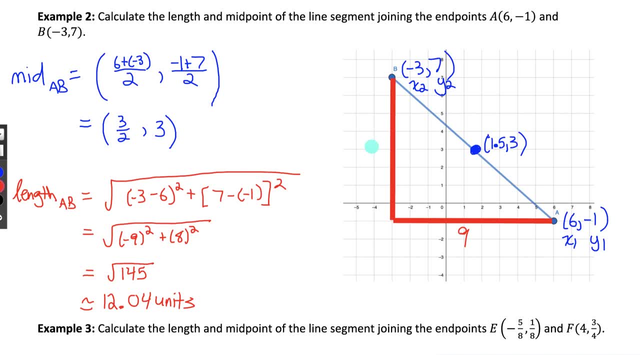 and i found out that the length of the vertical component is eight. i got that by doing the difference in the y coordinates of the endpoints and using pythagorean theorem we were able to solve for the length of the hypotenuse, which is line segment a- b. let's move on to example three. 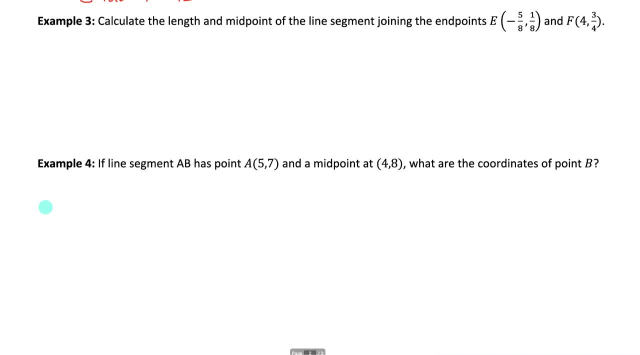 and this is going to be the first one where i haven't given you a diagram, and actually i didn't give you very much room to work here, so i'll write small. we're going to find the length and midpoint of the line segment joining e and f. i noticed the x and y coordinates of my endpoints. 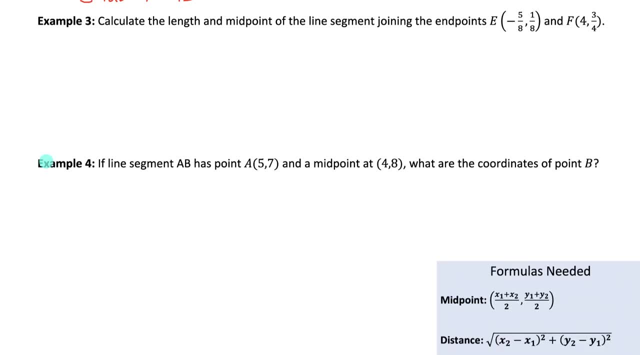 have some fractions involved, but if we follow the same formulas and as long as you know the rules for working with fractions, we can solve this question the same way we did the previous two. i'll find the midpoint of e- f, and maybe it'll be helpful for me to label these points as my. 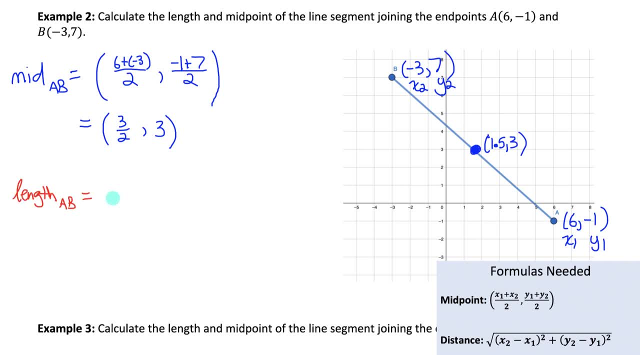 To find the length of line segment AV and to find the length we need to square root the difference in the x's squared plus the difference in the y's squared. So we'll do the difference in the x coordinates and we'll follow what the formula tells us to do. We'll 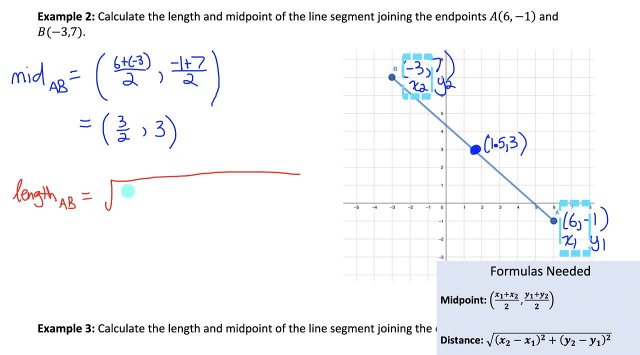 do x2 minus x1, so negative 3 minus 6, squared plus the difference in the y coordinates. And the formula says to do y2 minus y1, so I will do 7 minus negative 1. squared, If I simplify underneath the square root I would have negative 9, squared plus. 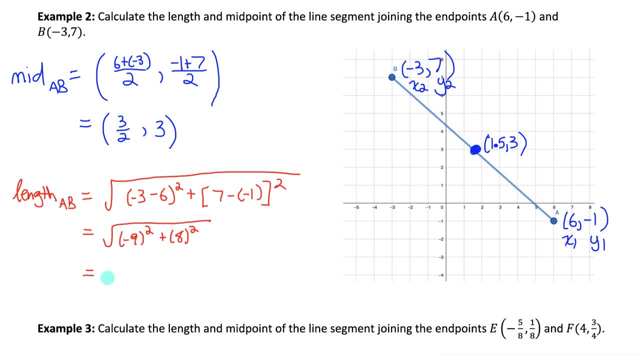 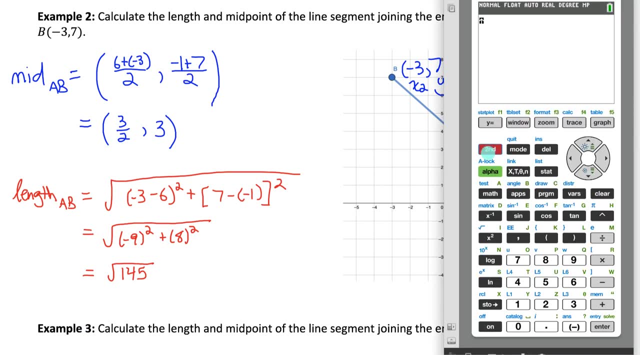 8 squared. If I collect those terms under the square root, I would have the square root of 145 as my exact answer. If I want an approximate answer, I can type that on my calculator and I get approximately 12.04 units. 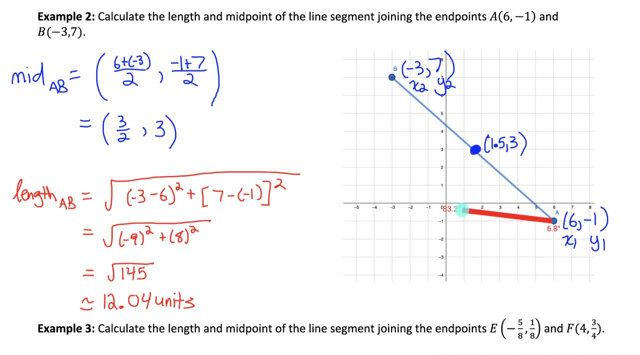 And hopefully you remember why I did that. I hope you did. Thanks for watching. I'll see you next time. This is why that formula works Really. what we did was we used Pythagorean theorem, by turning this into a right triangle And by finding the difference in the x coordinates. 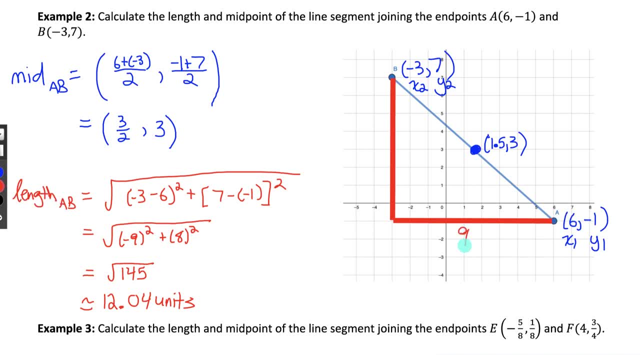 we found out that the length of the horizontal component is nine units. I get that from the absolute value of the difference of the x's. And I found out that the length of the vertical component is eight. I got that by doing the difference in the y coordinates of the endpoints. 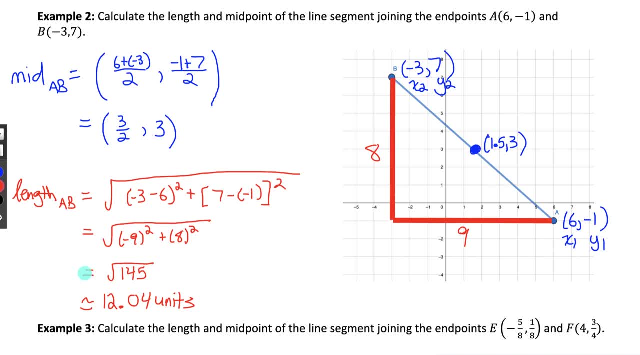 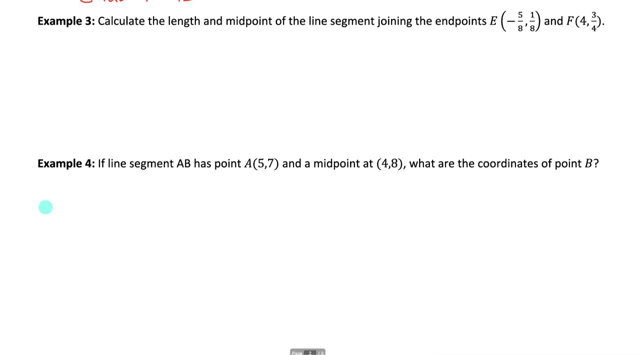 And using Pythagorean theorem, we were able to solve for the length of the hypotenuse is line segment a, b. let's move on to example three, and this is going to be the first one where i haven't given you a diagram, and actually i didn't give you very much room to work here, so i'll write. 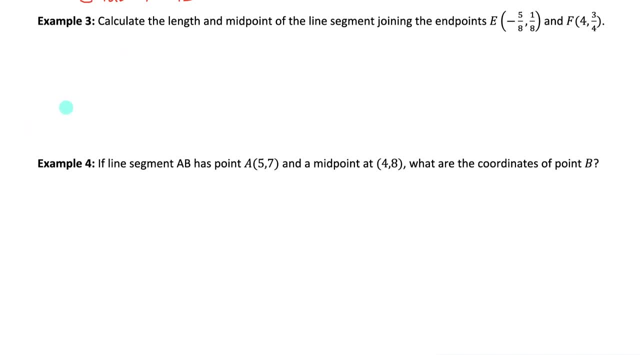 small. we're going to find the length and midpoint of the line segment joining e and f. i noticed the x and y coordinates of my endpoints have some fractions involved, but if we follow the same formulas and as long as you know the rules for working with fractions, we can solve this question. 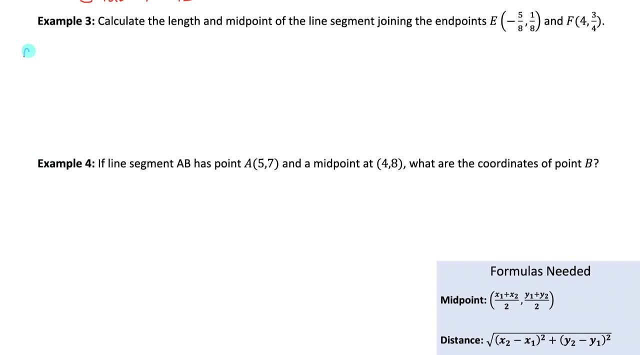 the same way we did the previous two. i'll find the midpoint of ef and maybe it'll be helpful for me to label these points as my first point. so i'll label e as x1, y1 and i'll make f my second point, x2, y2. if i follow my formula for midpoint, i need to average the x coordinates by adding. 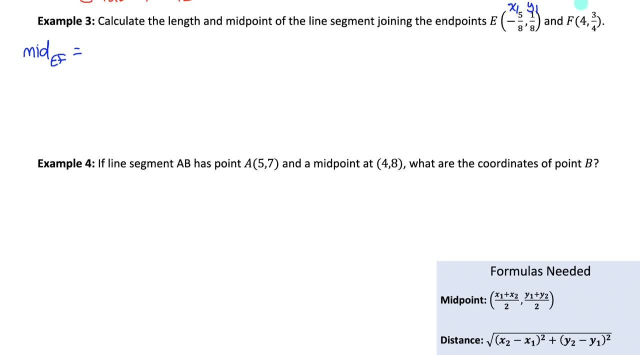 first point. so i'll label e as x1y1 and i'll make f my second point x2y2. if i follow my formula for midpoint, i need to average the x coordinates by adding them and dividing by 2, so i do negative 5 over 8 plus 4 over 2. that will get me the x coordinate of the x coordinate of the sub coordinate. 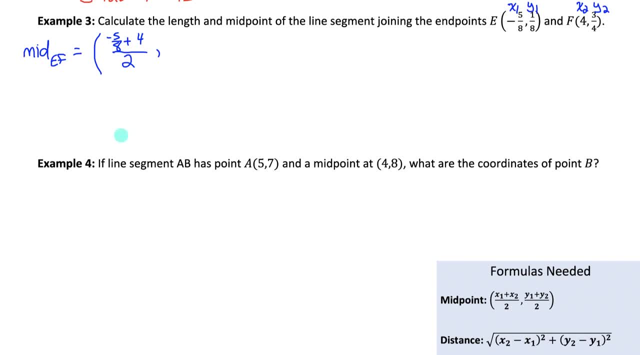 the midpoint. to get the y coordinate of the midpoint i need to find the average of the y coordinates of the endpoints. i'll do y1 plus y2 over 2. that's 1 over 8 plus 3 over 4 over 2.. 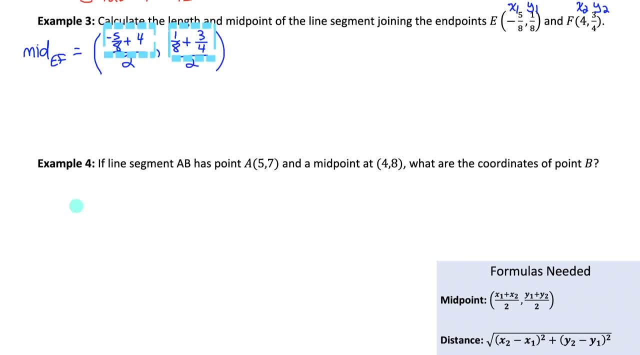 now notice, in the numerators of the x and y coordinates i have fractions being added. i'm going to need to get a common denominator, this 4. you can think of it as a 4 over 1. i need it to have a denominator of 8.. so i will multiply that 4 over 1, top and bottom by 8, to get an. 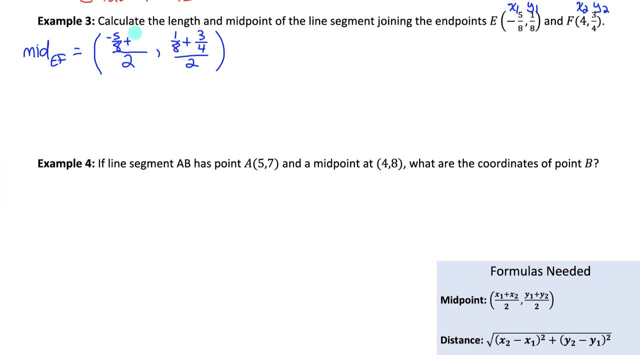 equivalent fraction that has a denominator of 8 and that gives me 32 over 8.. and if i look at the y coordinate of my midpoint, i look at the numerator also, fractions being added- my common denominator will be 8. so i'll multiply that 3 over 4, top and bottom by 2, so that it has a denominator. 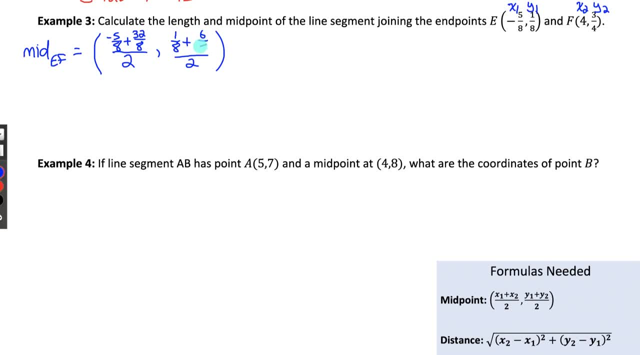 of 8. and that gives me an equivalent fraction of 6 over 8.. now that they have common denominators, i can add them. if i look at the x coordinate, negative 5 over 8 plus 32 over 8. the rule for adding fractions with a common denominator is to add the numerators. 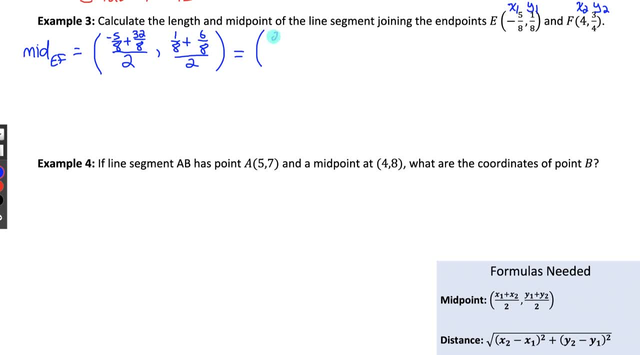 negative: 5 plus 32, which is 27, and keep the denominator, so i have 27 over 8 and keep in mind that is over 2 comma. the y coordinate: i have 1 over 8 plus 6 over 8, that is 7 over 8. 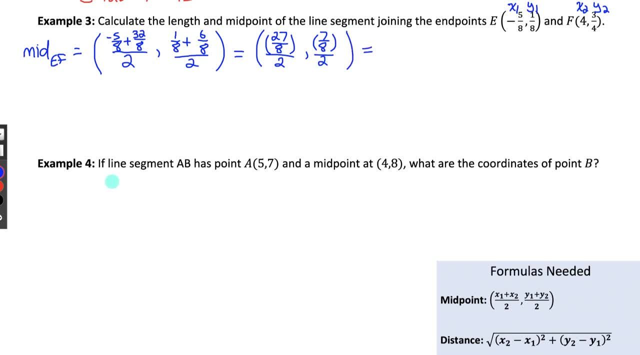 is also over 2.. i have two fractions and they're both being divided by 2.. to divide a fraction by a whole number, there is a shortcut. but for our first time it may be easier for me to rewrite those whole numbers of 2, to rewrite those as 2 over 1s. that way we've turned it into a fraction. 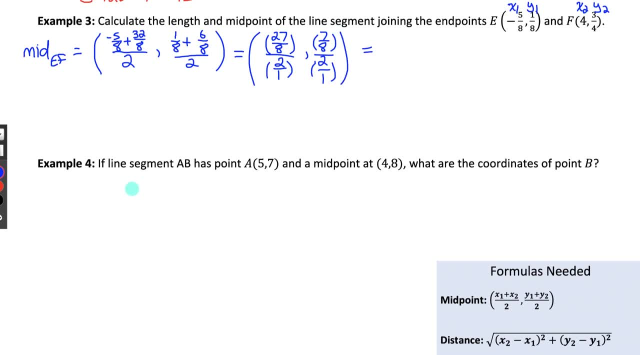 over a fraction. and when dividing fractions the rule is you flip and multiply. so the 27 over 8, we leave that as 27 over 8.. so the 27 over 8, we leave that as 27 over 8.. so the 27 over 8, we leave that as 27 over 8.. 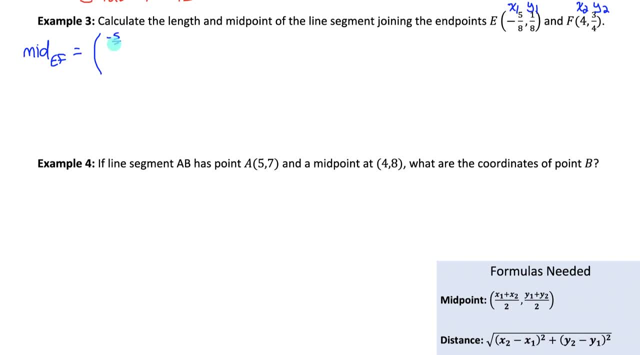 them and dividing by two. so i have to do negative five over eight plus four over two. that will get me the x coordinate of the midpoint. to get the y coordinate of the midpoint i need to find the average of the y coordinates of the endpoints. i'll do y1 plus y2 over two, that's. 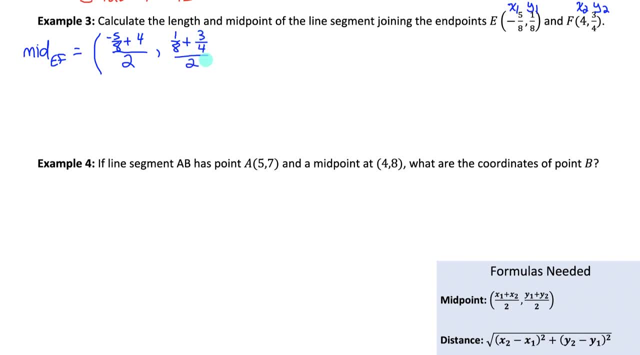 one over eight, plus three over four over two. now notice, in the numerators of the x and y coordinates i have fractions being added. i'm going to need to get a common denominator, this four. you can think of it as a four over one. i need it to have a denominator. 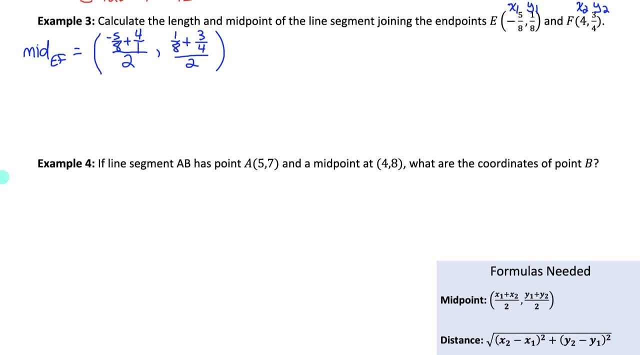 of eight. so i will multiply that four over one, top and bottom by eight, to get an equivalent fraction that has a denominator of eight and that gives me 32 over eight. and if i look at the y coordinate of my midpoint, i look at the numerator also, fractions being added. 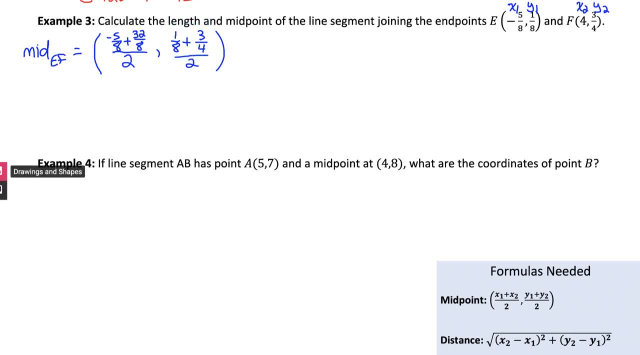 my common denominator will be eight. so i'll multiply that three over four, top and bottom by two, so that it has a denominator of eight, and that gives me an equivalent fraction of six over eight. now that they have common denominators, i can add them. if i look at the x coordinate, negative, 5 over 8 plus 32 over 8. the: 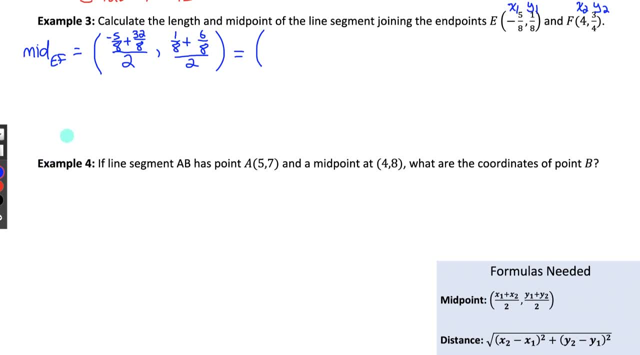 rule for adding fractions with a common denominator is to add the numerators negative 5 plus 32, which is 27, and keep the denominator. so i have 27 over 8 and keep in mind that is over 2 comma. the y coordinate. i have 1 over 8 plus 6 over 8, that is 7 over 8 and that is also over. 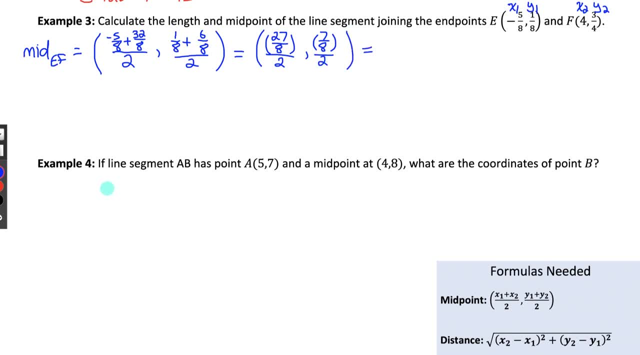 2.. i have two fractions and they're both being divided by 2.. to divide a fraction by a whole number there is a shortcut, but for our first time it may be easier for me to rewrite those whole numbers of 2, to rewrite those as 2 over 1s. that way we've turned it into a fraction over a fraction. 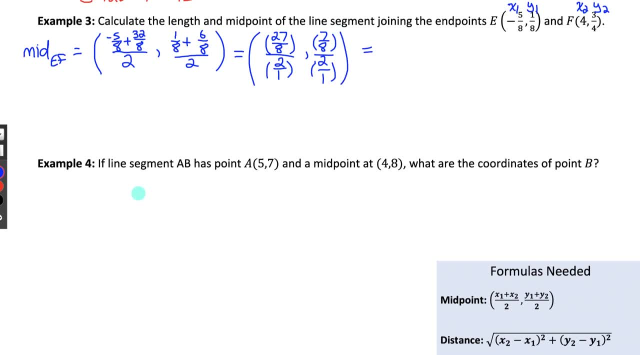 and when dividing fractions the rule is you flip and multiply. so the 27 over 8, we leave that as 27, but we change it to multiply and multiply by the reciprocal of the fraction in the denominator. so the reciprocal of 2 over 1 is 1 over 2.. that will give me the x coordinate and then the y. 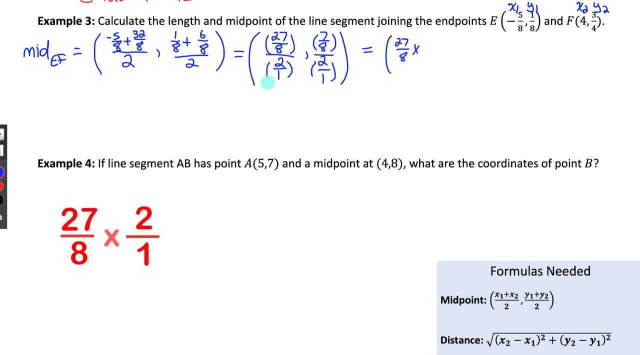 but we change it to multiply, and multiply by the reciprocal of the fraction in the denominator. so the reciprocal of 2 over 1 is 1 over 2.. that will give me the x coordinate and then the y coordinate. do the same. leave the 7 over 8 times the reciprocal of the fraction in the denominator. 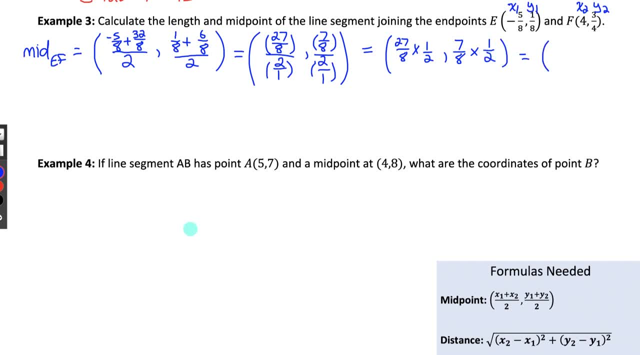 which is 1 over 2.. and now that it's written as multiplication, multiplying fractions is easy. just multiply the numerators 27 times 1 is 27, and multiply the denominators 8 times 2 is 16.. looking at the y coordinate: 7 times 1 is 7 and 8 times 2 is 16.. so the midpoint is 27 over 16. 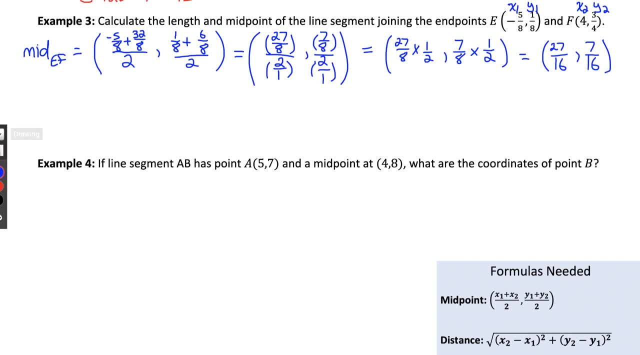 comma 7 over 16.. now i said there was a shortcut. let me just rewrite the middle step here the way we originally had it. if you notice, when you have a fraction being divided by a whole number, the denominator of the fraction just gets multiplied by the whole number, 8 times 2. 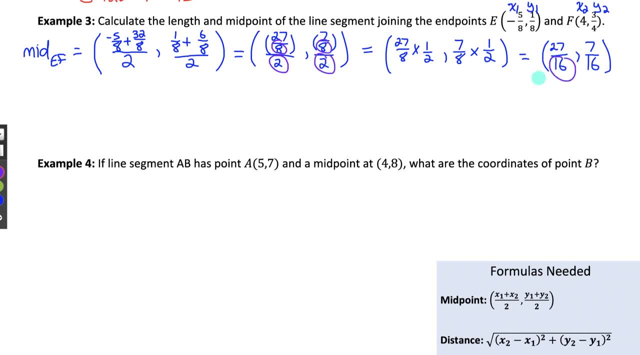 16.. and same thing with the y coordinate: 8 times 2: 16.. so that's a little shortcut if you want to use that, if you have a fraction being divided by a whole number. let's now find the length. remember to find the length i need to do the square root of. 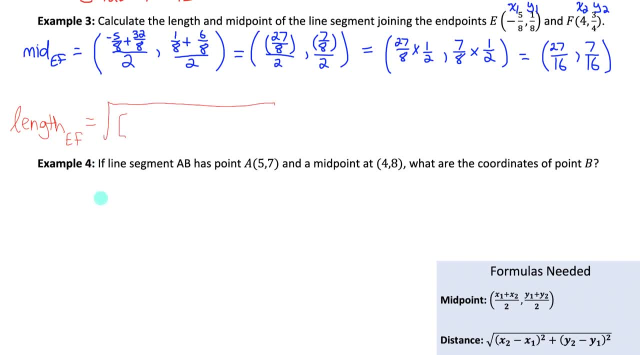 the difference in the x coordinates. so i will need to do x 2 minus x 1 squared, that's 4 minus negative, 5 over 8 squared, plus the difference in the y coordinate squared. if i do y 2 minus y 1, that's 3 over 4 minus 1 over 8 squared. now i already know how to get common denominators here. 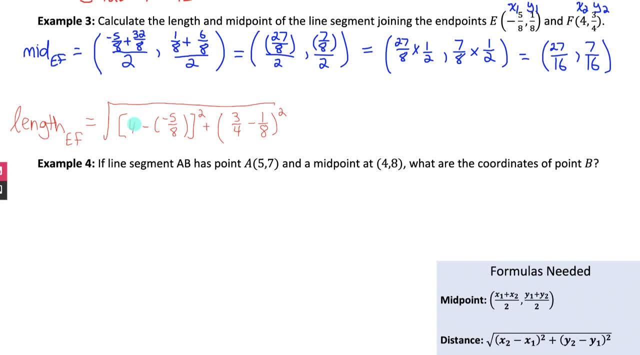 when i'm subtracting fractions, i also need common denominators. so i'm going to change that 4 to a 32 over 8, and i'm going to change this 3 over 4 to a 6 over 8.. and now, if i simplify the rule for: 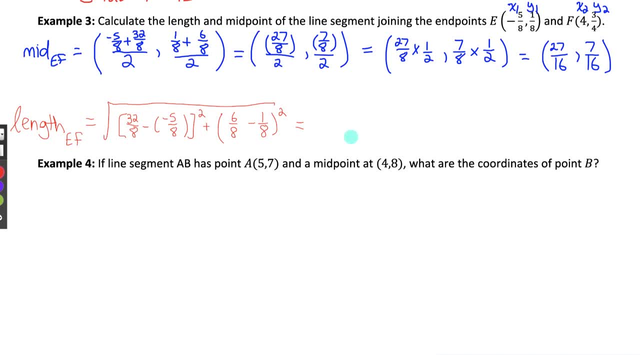 subtracting fractions is the same as for adding. we just subtract the numerators and leave the denominators the same. to leave the denominator the same over 8 minus negative, 5 over 8 would be 37 over 8, and 6 over 8 minus 1 over 8 is 5 over. 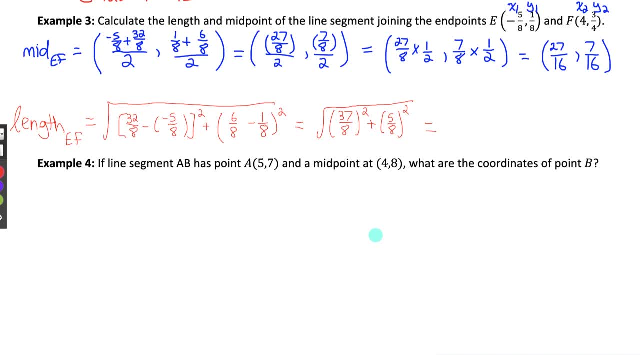 8. When you have an exponent on a fraction you need to apply that exponent to the numerator and denominator. So I would need to square the 37 and the 8 in the first fraction. That would be 1,369 over 64, plus. if I do the same thing to the second fraction, square. 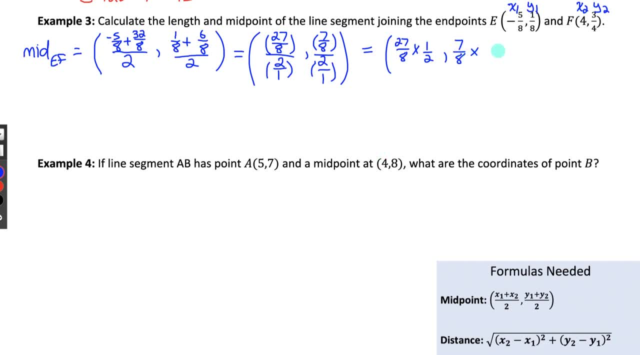 coordinate. do the same. leave the 7 over 8 times the reciprocal of the fraction in the denominator, which is 1 over 2.. and now that it's written as multiplication, multiplying fractions is easy. just multiply the numerators 27 times 1 is 27, and multiply the denominators 8 times 2 is 16.. 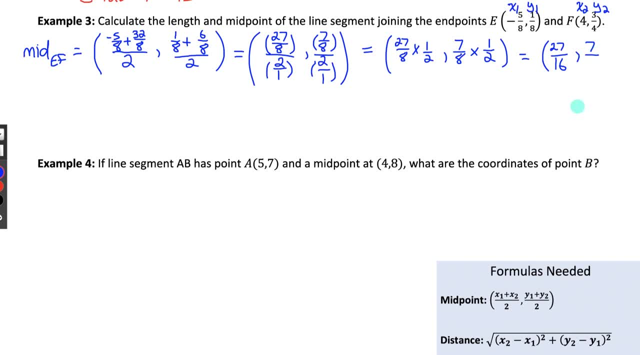 looking at the y coordinate, 7 times 1 is 7 and 8 times 2 is 16.. so the midpoint is 27 over 16, comma 7 over 16.. now i said there was a shortcut. let me just rewrite the middle step here, the. 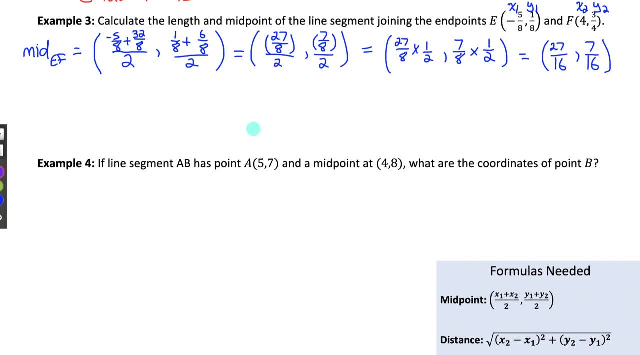 way we originally had it. if you notice, when you have a fraction being divided by a whole number, the denominator of the fraction just gets multiplied by the whole number: 8 times 2- 16.. and same thing with the y coordinate: 8 times 2. 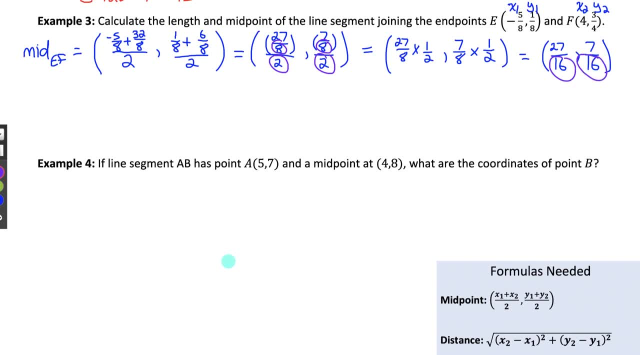 16. So that's a little shortcut if you want to use that. if you have a fraction being divided by a whole number, Let's now find the length. Remember, to find the length I need to do the square root of the difference in the x coordinates. So I will need to do x, two minus. 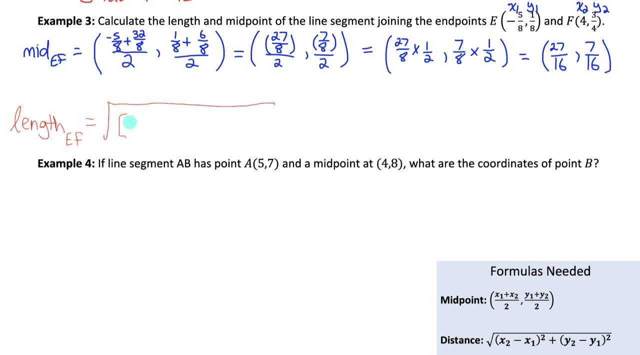 x one squared, that's four minus negative five over eight squared, plus the difference in the y coordinate squared. If I do y two minus y one, that's three over four minus one over eight squared. Now I already know how to get common denominators here. when 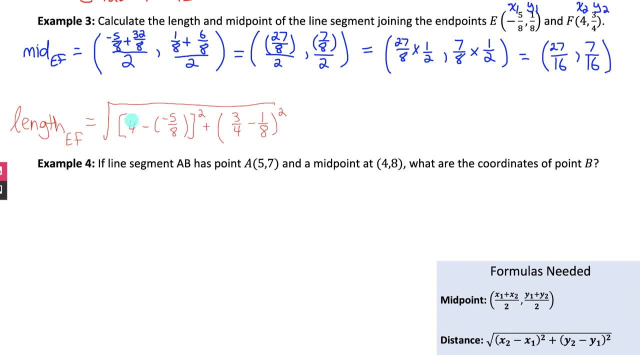 I'm subtracting fractions, I also need common denominators. So I'm going to change that four to a 32 over eight And I'm going to change this three over four to a six over eight. And now, if I simplify, the rule for subtracting fractions is the same as for adding. 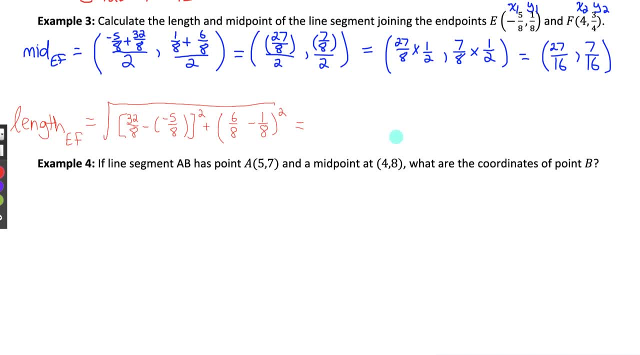 we just subtract the numerator And leave the denominator the same. 32 over eight minus negative. five over eight would be 37 over eight, And six over eight minus one over eight is five over eight. When you have an exponent on a fraction, you need to apply that exponent to the numerator and denominator. 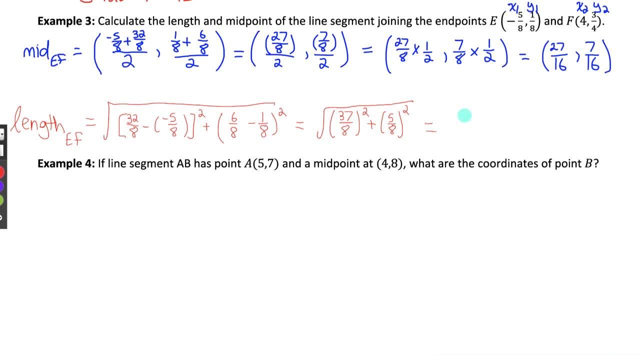 So I would need to square the 37 and the eight in the first fraction, that would be 1369 over 64. Plus, if I do the same thing to the second fraction, squared the numerator and denominator five squared, is 25, over eight squared, which is 64. And now I can get an. 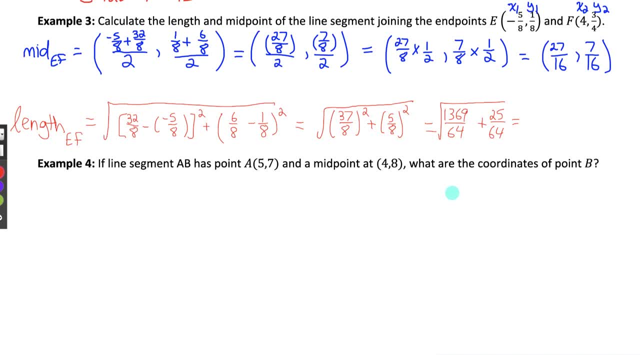 exact answer expressed as a fraction. they already have a common denominator. So if I add the numerators, that would be 1394.. Keep the denominator the same. Here's an exact answer. Now that fraction could be reduced, But for our purposes, for this, that's fine. 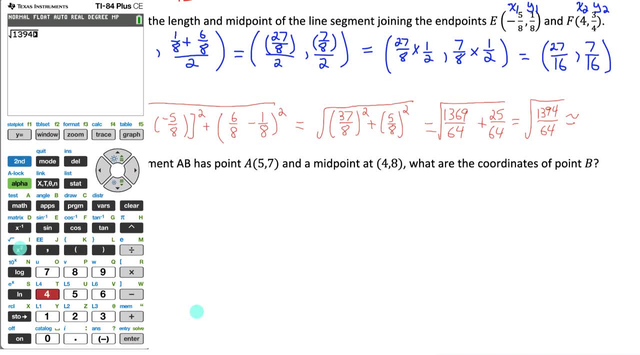 If we want an approximate answer. I can evaluate that on my calculator and I get about 4.6.5.. So I'm going to add that to the numerator and I'm going to add that to the denominator. and I'm going to add that to the denominator and I'm going to add that to the denominator. 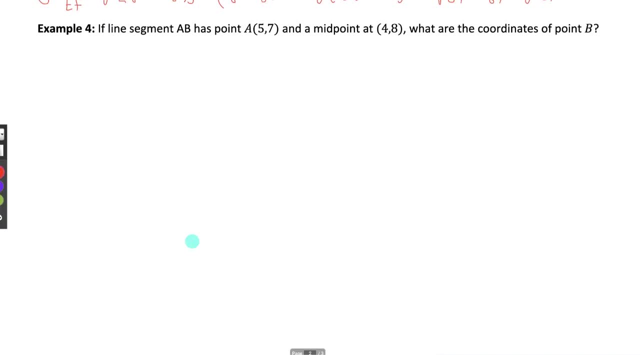 plus nine plus seven units. right, there are two more examples left to do. The next one is a little bit different. It says: if lineseg A- B has point a at five, seven and midpoint for a, what are the coordinates of point B? So this one's different because for 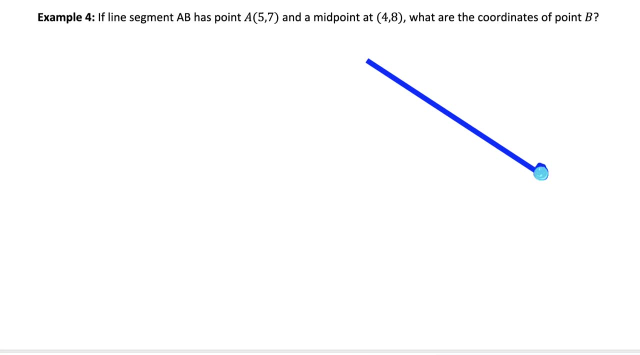 our line segment. I know one of the endpoints. We'll call this one here, a. I know that's at five seven. I don't know the other endpoint. I don't know Point B. point B: I'm not sure what the coordinates of that point are. So I don't know what x and y are. 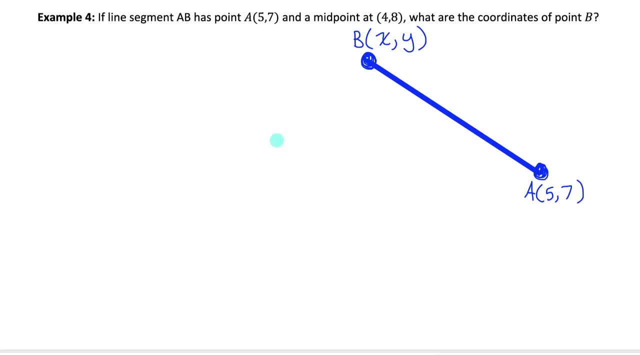 for that point, But I do know what the midpoint is. It tells me that the midpoint is at 4, 8.. So our job in this question is to solve, for what are the x and y coordinates of endpoint B? Now it may help if I choose whether B is going to be my first or second point, and same with A. 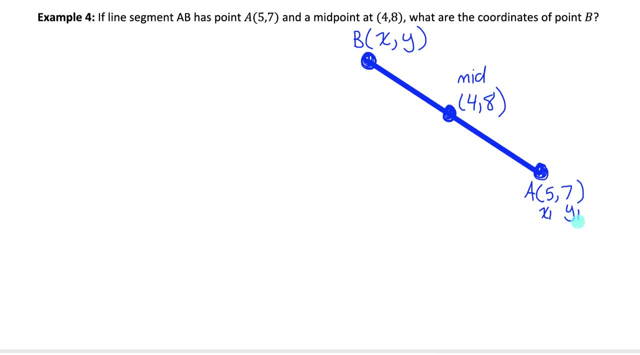 I'll say: A is my first point, my x1 y1.. Therefore, B is my second point, So it's my x2- y2.. And now, if I follow my formula for midpoint, I know that the midpoint, which is 4, 8, must be equal to. 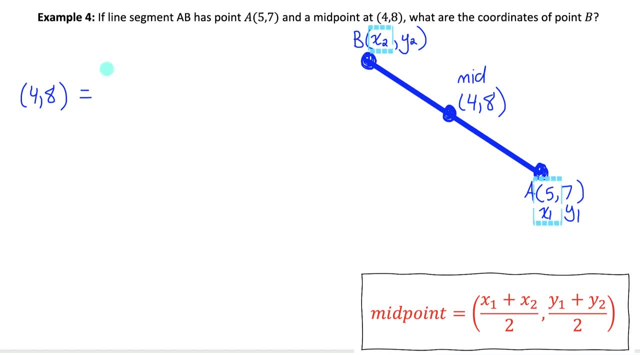 the average of the x coordinates of the endpoints, And I get the average of them by adding them and dividing by 2.. So x1,, which is 5,, plus x2, which we don't know over 2.. And the y coordinate of: 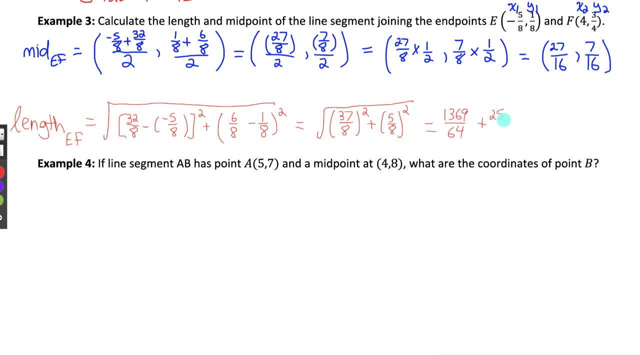 the numerator and denominator. 5 squared is 25 over 8 squared, which is 64.. And now I can get an exact answer expressed as a fraction. They already have a common denominator. So if I add the numerators, that would be 1394.. Keep the denominator the same. Here's an exact 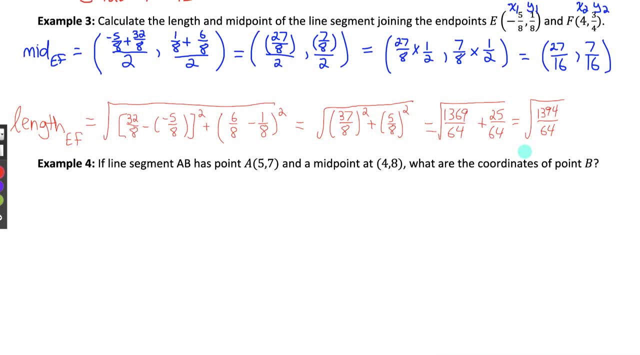 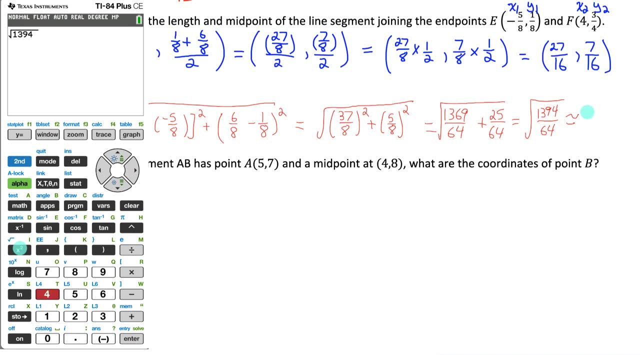 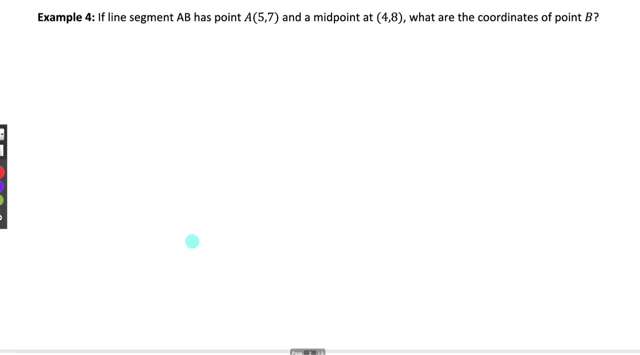 answer. Now that fraction could be reduced, but for our purposes, for this, that's fine. If we want an approximate answer, I can evaluate that on my calculator And I get about 4.6 units. Alright. there are two more examples left to do. The next one's a little bit different. 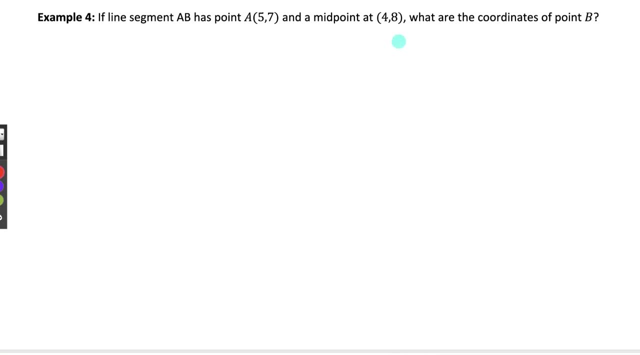 It says: if line segment AB has point A at 5, 7 and midpoint 4, 8, what are the coordinates of point B? So this one's different, because for our line segment I know one of the endpoints. We'll call this one here- A. I know that's at 5, 7.. I don't know the other endpoint. 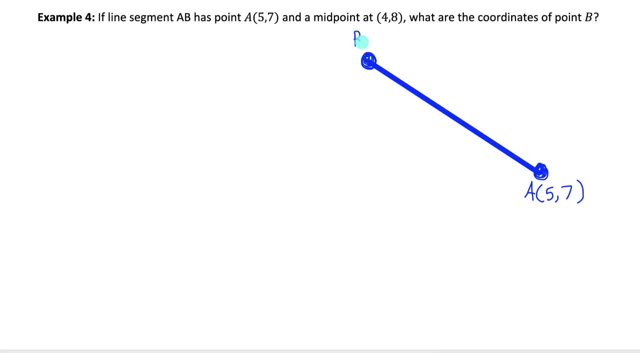 I don't know point B, point B, I'm not sure what the coordinates of that point are, So I don't know what x and y are for that point. But I do know what the midpoint is. it tells me that the midpoint 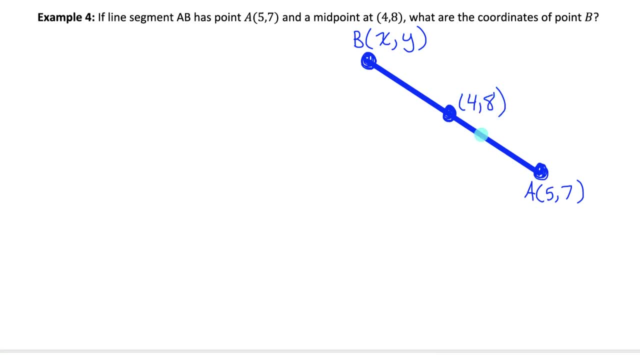 is at 48.. So our job in this question is to solve for what are the x and y coordinates of endpoint B? Now it may help if I choose whether B is going to be my first or second point, and same with a. I'll say a is my first point, my x1, y1. Therefore, B is my second. 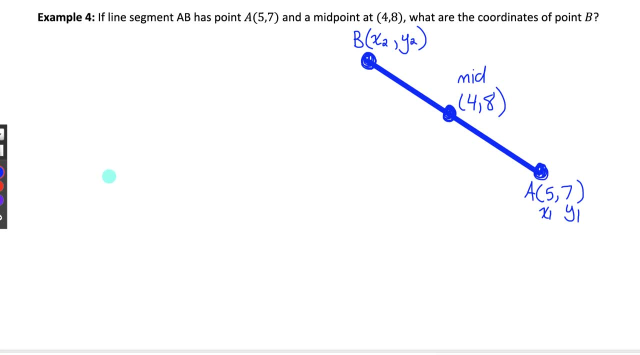 point. So it's my x2, y2.. And now, if I follow my formula for midpoint, I know that the midpoint, which is 48, must be equal to the average of the x coordinates of the endpoints. And I get the average of them by adding them and dividing by two. So x1, which is five plus. 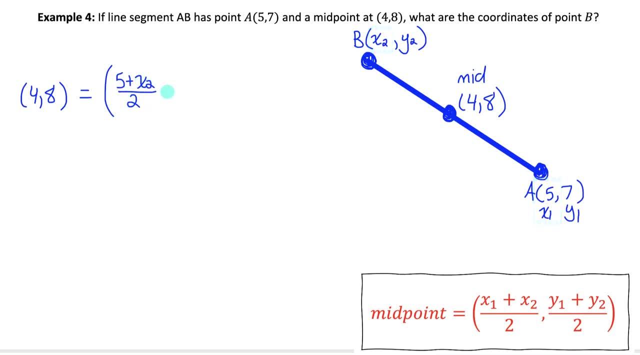 x2, which we don't know, over two And y coordinate of the midpoint. we would get by averaging the y coordinates of the endpoints, y1 plus y2, which is 7 plus y2. we're not sure what that is. divide by 2 to find the average of them. 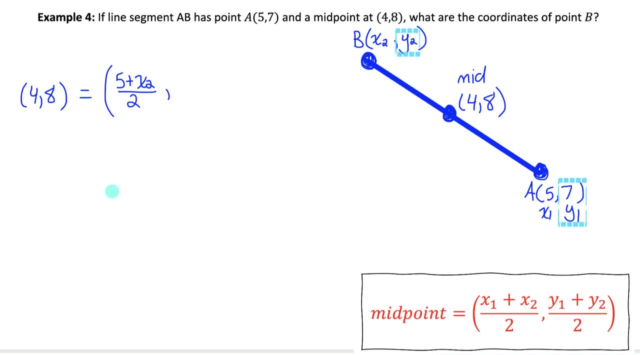 the midpoint we would get by averaging the y coordinates of the endpoints, y1 plus y2, which is 7 plus y2, we're not sure what that is. Divide by 2 to find the average of them. Now let's separate this into two equations. One for the x coordinate of the midpoint. 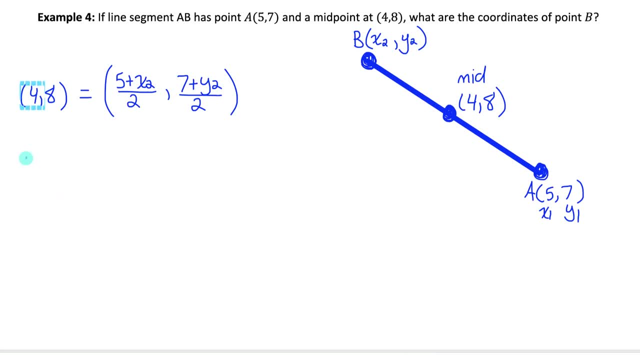 one for the y coordinate. The x coordinate of the midpoint is 4, and that's obtained by adding the x coordinates of the endpoints and dividing by 2.. And the y coordinate of the midpoint 8.. be equal to the average of the y coordinates of the endpoints, 7 plus y2 over 2.. i now have 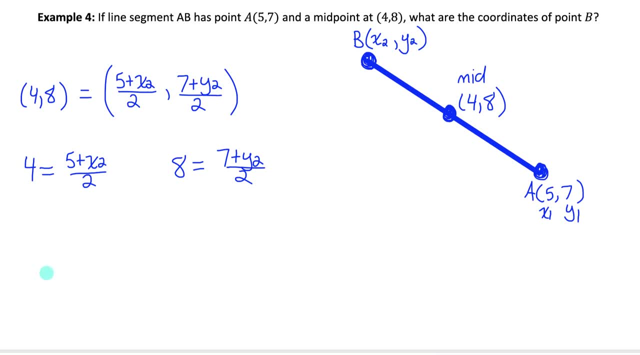 two equations. i can solve each of these equations for the one unknown in each of them, the first thing i would do to isolate the variable is move the divided by 2 to the other side by doing the inverse operation, which is multiplying by 2.. 4 times 2 is 8. so i have 8 equals 5 plus x2. and if 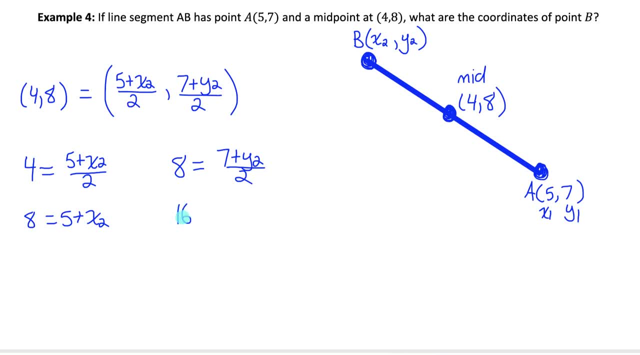 i'm looking at the y coordinate equation: 8 times 2 is 16, so i have 16 equals 7 plus y2. and now in each of them i just have one step left to isolate the variable. for the x coordinate, i'll just subtract the 5 to the other side and i would have x: 2 equals 8 minus 5, which is 3. and to isolate y2, 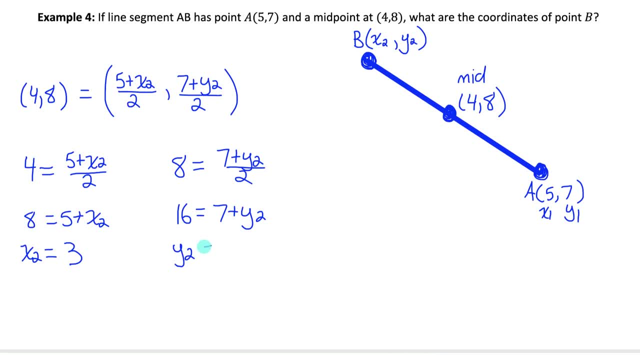 i seem to subtract the 7 to the other side and i would get y2 equals 16 minus 7, which is 9.. so i've now discovered that the coordinates of b are actually 3 and 9.. and this makes sense because if i were to look at the x coordinates, 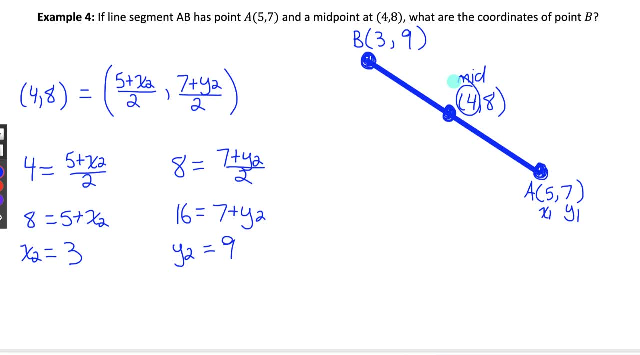 of the endpoint 3 and 5, of course 4 is in the middle of 3 and 5.. if i look at the y coordinates- 9 and 7- of course 8 is in the middle of 9 and 7.. so it appears we have the correct. 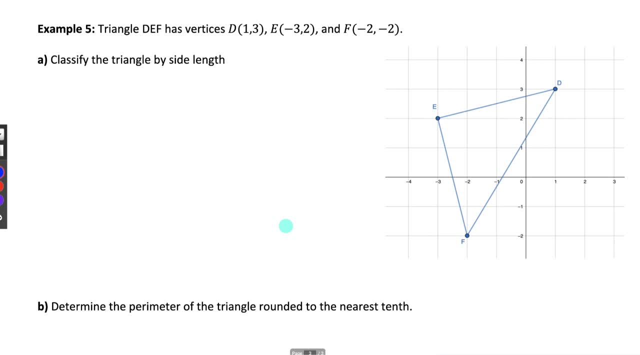 coordinates of endpoint b. our last question, example 5 says we have triangle d, e, f and it gives us the coordinates of the vertices of that triangle and it asks us to, in part a, class classify the triangle by side length. so i'm going to need to know the length of all three sides of 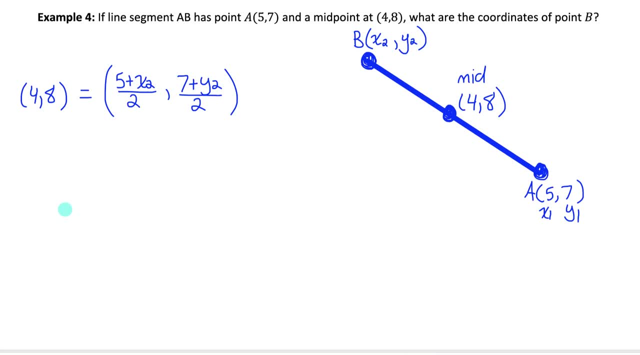 now let's separate this into two equations, one for the x coordinate of the midpoint, one for the y coordinate. the x coordinate of the midpoint is 4, and that's obtained by adding the x coordinates of the endpoints and dividing by 2, and the y coordinate of the midpoint, 8, should be equal. 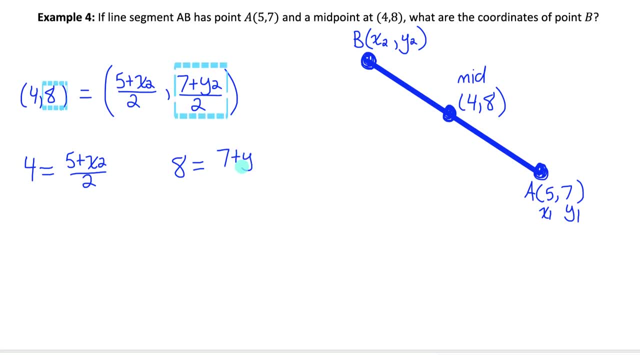 to the average of the y coordinates of the endpoints 7 plus y2 over 2.. i now have two equations. i can solve each of these equations. for the one unknown in each of them, the first thing i would do to isolate the variable is move the divided by 2 to the other side by doing the. 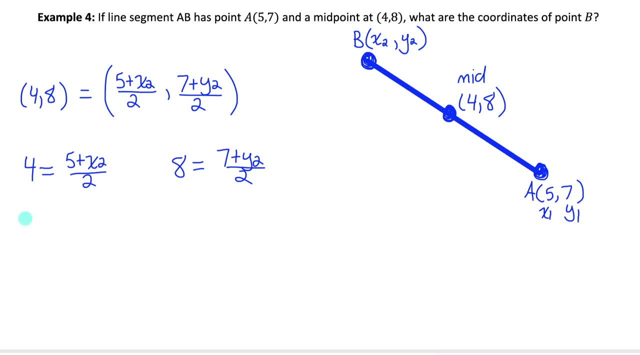 inverse operation, which is multiplying by 2.. 4 times 2 is 8, so i have 8 equals 5 plus x2. and if i'm looking at the y coordinate equation, 8 times 2 is 16, so i have 16 equals 7. 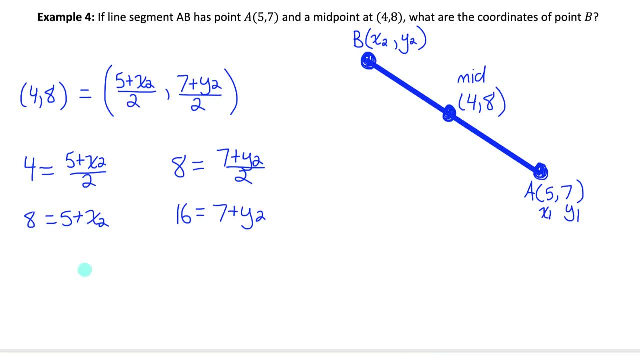 plus y2. and now in each of them i just have one step left. to isolate the variable for the x coordinate, i'll just subtract the 5 to the other side and i would have x 2 equals 8 minus 5, which is 3. and to isolate y2, i seem to subtract the 7 to the other side. 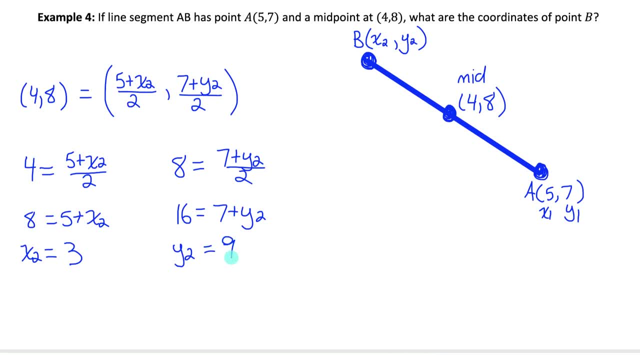 and i would get. y2 equals 16 minus 7, which is 9.. so i'm now discovered that the coordinates of B are actually 3 and 9.. And this makes sense because if I were to look at the x coordinates of the endpoint 3 and 5, of course 4 is in the middle of 3 and 5.. 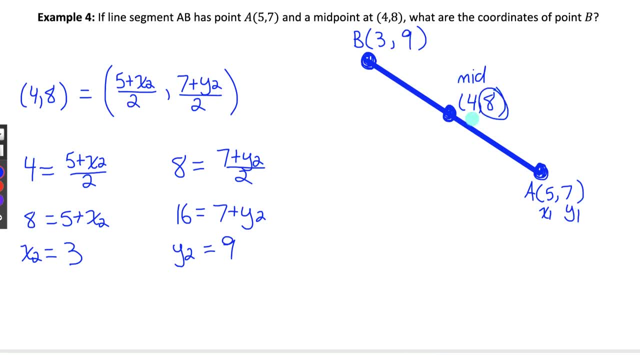 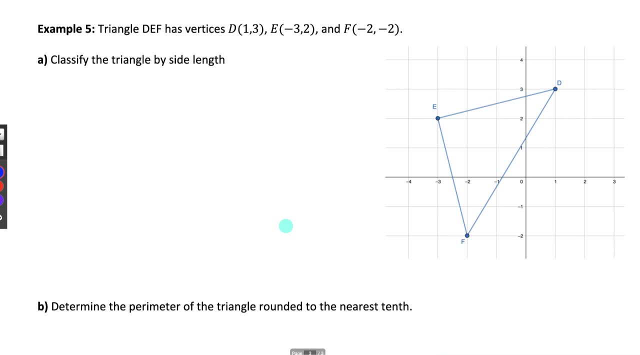 And if I look at the y coordinates- 9 and 7,, of course 8 is in the middle of 9 and 7.. So it appears we have the correct coordinates of endpoint B. Our last question, example 5, says we have: 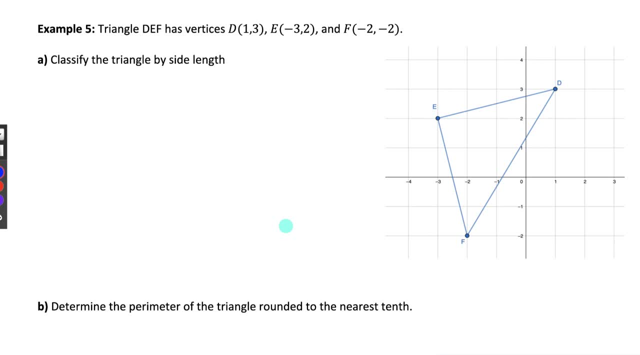 triangle D, E, F, and it gives us the coordinates of the vertices of that triangle And it asks us to, in part A, classify the triangle by side length. So I'm going to need to know the length of all three sides of this triangle to decide whether this triangle is scalene isosceles. 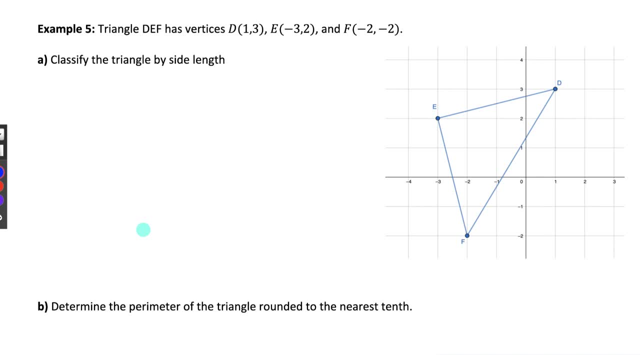 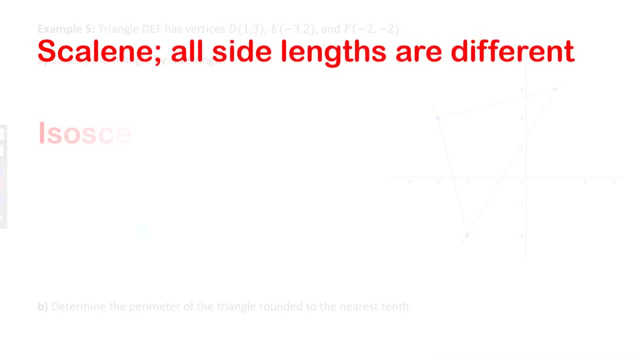 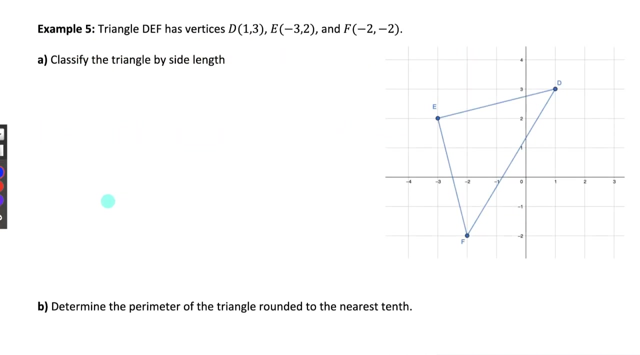 this triangle. to decide whether this triangle is scalene, isosceles or equilateral, if all three side lengths are different, it would be scalene. if two of the side lengths are equal, it's isosceles. if all three side lengths are equal, then it's equilateral. so let's find the length of all. 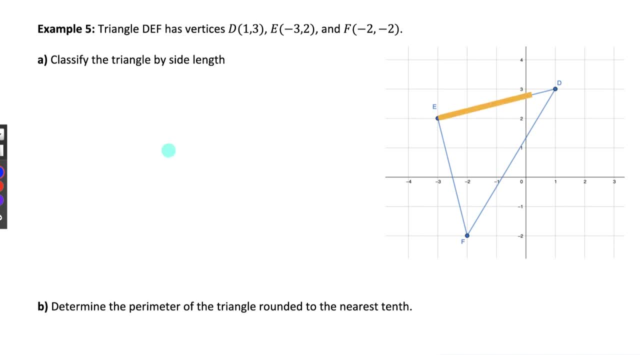 three sides. let's start by finding the length of e- d. let me label the coordinates for e and d and i'll choose point e to be my first point, my x1- y1. point d to be my second point, my x2, y2. and now 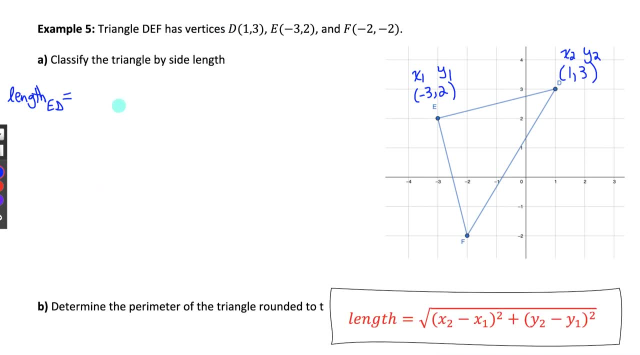 i'll go ahead and follow the length formula which tells me to do the square root of the difference in the x coordinate squared, so 1 minus negative, 3 squared, plus the difference in the y coordinate squared, 3 minus 2 squared. if i simplify, under the square root the difference in the x coordinates is: 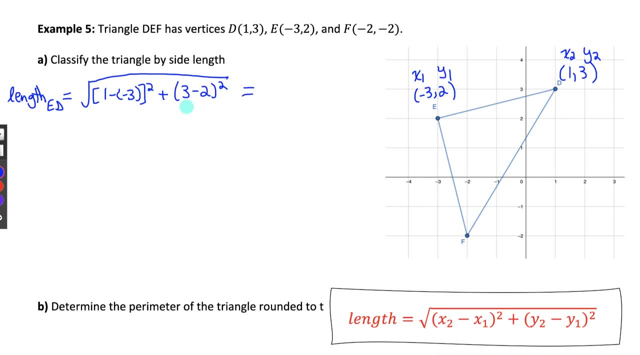 4 squared is 16 plus the difference in the y coordinates is 1: 1 squared is 1, so 16 plus 1 is 17. therefore the length of line segment ed is root 17.. i'm not interested in the approximate value. 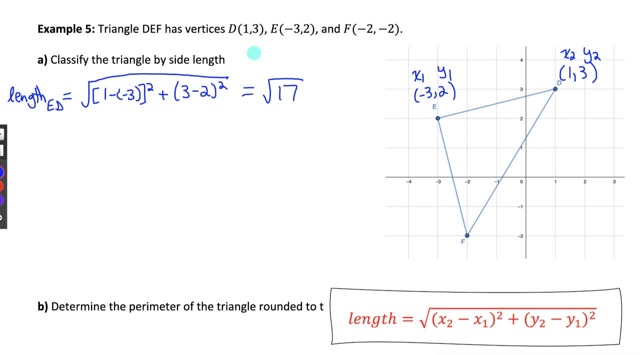 of this, it's four point: something having the exact value will be better. actually, when we're trying to classify this based on side length, let's now do the length of one of the other sides. let's do ef, so i'll make f. i'll label that point negative. 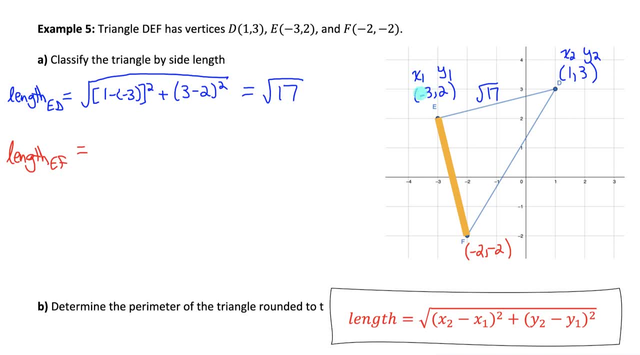 two, negative two. since i already have e as my first point, x1, y1, i'll just leave those labels and make f my second point, my x2, y2, and if i follow the length formula, i'll do the square root of the difference in the x coordinates squared: x2 minus x1 would be negative: 2 minus. 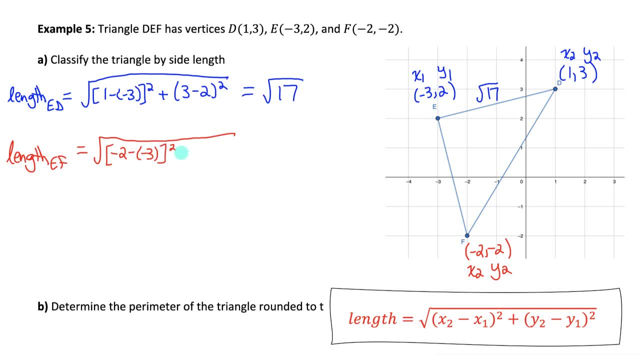 negative 3 squared plus the difference in the y coordinate squared. y2 minus y1 would be negative 2 squared. simplifying underneath the square root, the difference in the x's is 1. the difference in the y's is negative 4.. 1 squared plus negative 4 squared is once again root 17.. so those two. 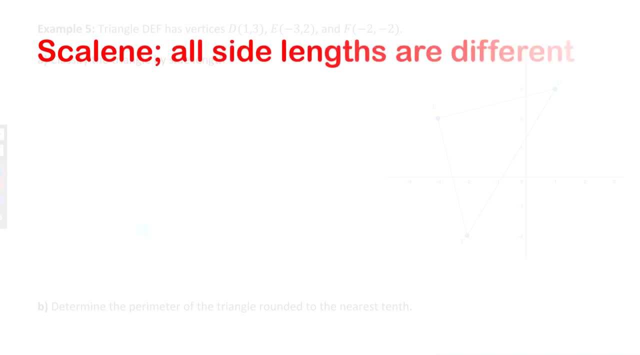 or equilateral. If all three side lengths are different, it would be scalene. If two of the side lengths are equal, it's isosceles. If all three side lengths are equal, then it's equilateral. So let's. 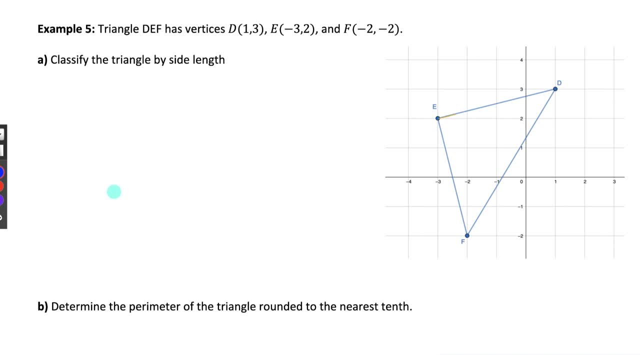 find the length of all three sides. Let's start by finding the length of E- D. Let me label the coordinates for E and D And I'll choose point E to be my first point, my x1, y1.. Point D to be 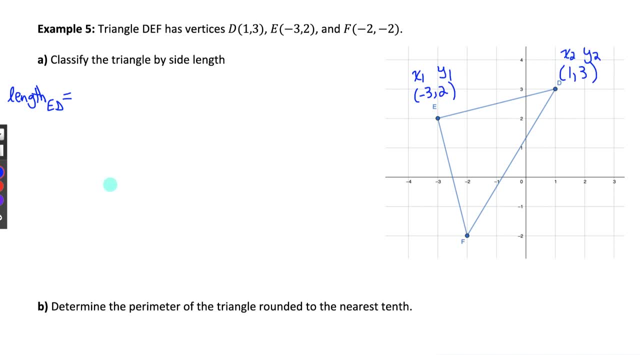 my second point, my x2, y2.. And now I'll go ahead and follow the length formula which tells me to do the square root of the difference in the x coordinates squared. so 1 minus negative 3 squared plus the difference in the y coordinates squared. 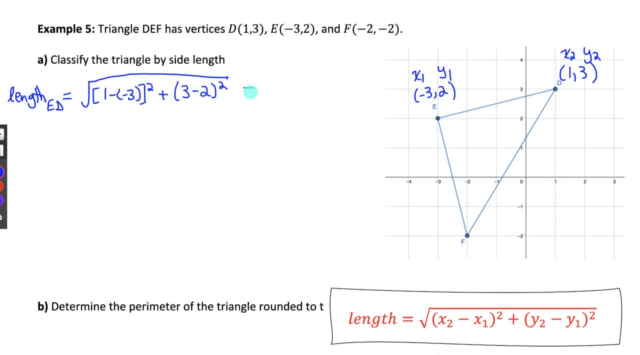 3.. 3 minus 2 squared. If I simplify, under the square root the difference in the x coordinates is 4, squared is 16, plus the difference in the y coordinates is 1.. 1 squared is 1,, so 16 plus 1. 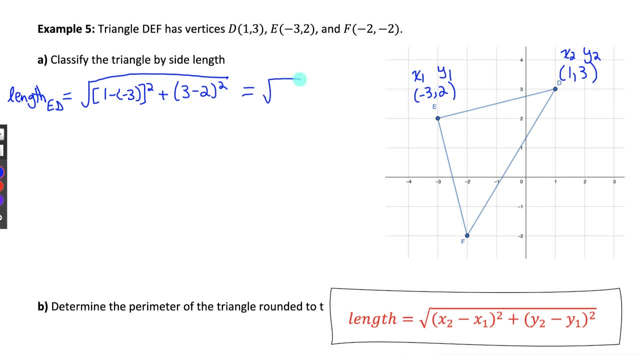 is 17.. Therefore, the length of line segment E D is root 17.. I'm not interested in the approximate value of this. It's 4 point. something Having the exact value will be better, actually, when we're trying to classify this based on side length, Let's now do: 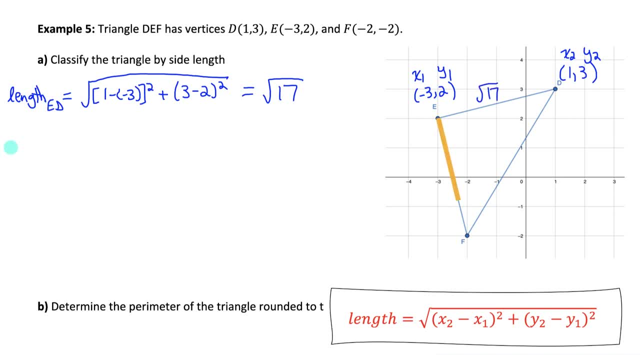 the length of one of the other sides. Let's do E, F, So I'll make F. I'll label that point negative 2,, negative 2.. Since I already have E as my first point- x1,, y1, I'll just leave those labels and 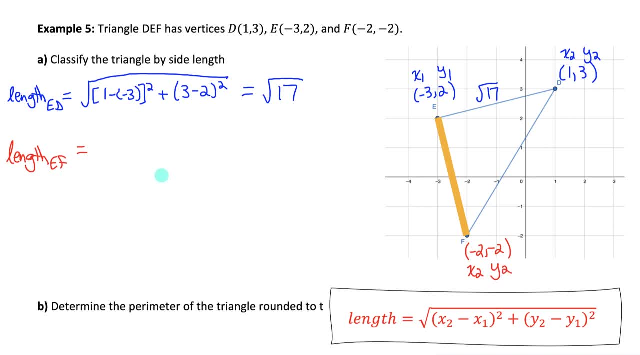 make F, my second point, my x2, y2.. And if I follow the length formula, I'll do the square root of the difference in the x coordinates squared. x2 minus x1 would be negative. 2 minus negative 3 squared. 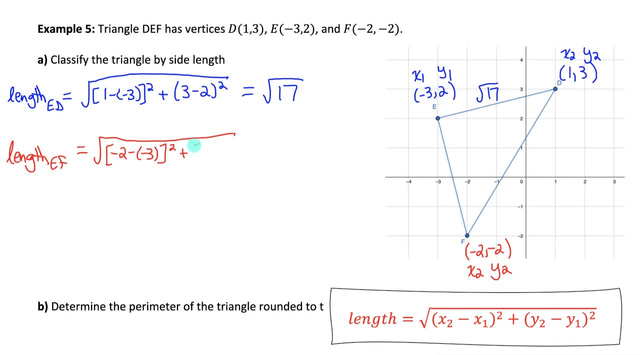 plus the difference in the y coordinates. squared, y2 minus y1 would be negative: 2 minus 2 squared. Simplifying underneath the square root, the difference in the x's is 1, the difference in the y's is negative, 4.. 1 squared plus negative 4 squared is once again root 17.. So those two 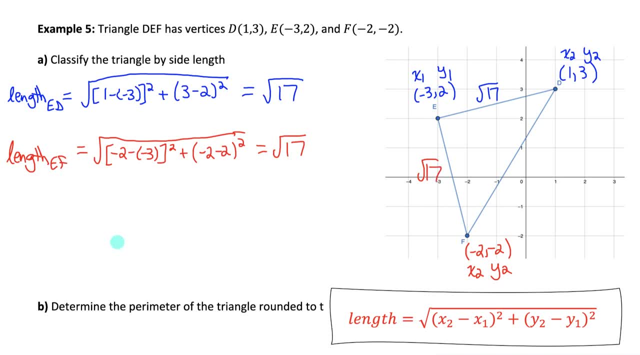 side lengths are the same. So this triangle is not scalene. it's either isosceles or equilateral. That will depend on what the length of line segment D F is. For line segment D F, I suppose D should be my first point, So I'll have to. 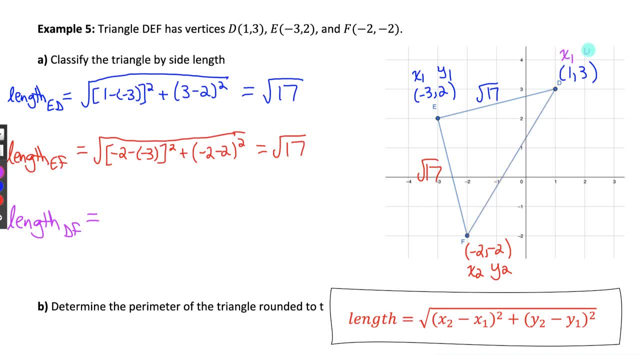 change those labels to make this x1, y1. And I already have F labeled x2, y2.. Following the length formula I do, the square root of the difference in the x coordinates squared. x2 minus x1 would be negative: 2 minus 1 squared plus the difference in the y coordinates. 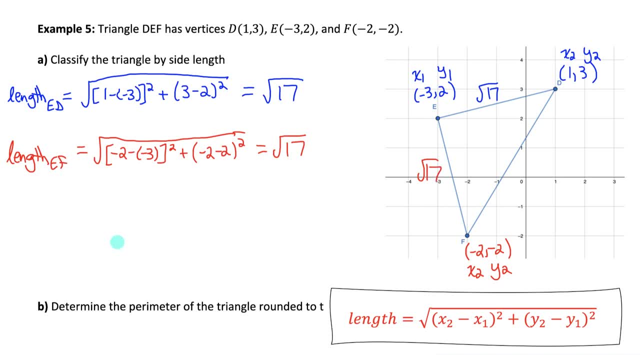 side lengths are the same, so this triangle is not scalene. it's either isosceles or equilateral. that will depend on what the line, the length of line segment df, is. for line segment df, i suppose d should be my first point. so i'll have to change those labels to make this x1- y1 and i already have f labeled x2- y2. 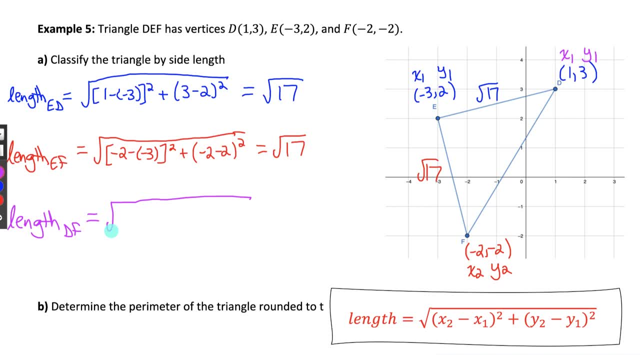 following the length formula, i do. the square root of the difference in the x coordinates, squared x2 minus x1 would be negative 2 minus 1 squared. plus the difference in the y coordinates, squared y2 minus y1, would be negative 2 minus 3 squared. simplifying underneath the square root of y2- y1 would be negative 2 minus 3 squared. 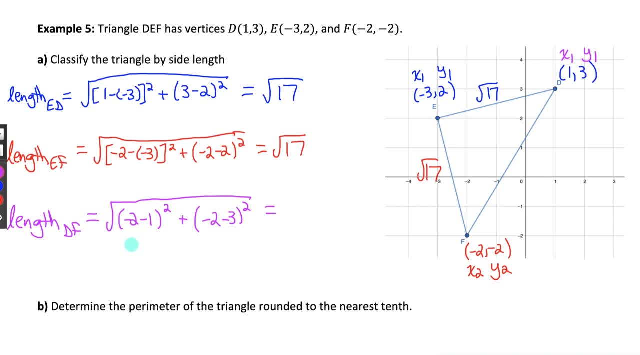 the difference in the x's is negative 3. the difference in the y's is negative 5. negative 3 squared plus negative 5 squared is 34.. so this would be the square root of 34.. now that i know that two sides of this triangle are equal, i can classify this as an isosceles. 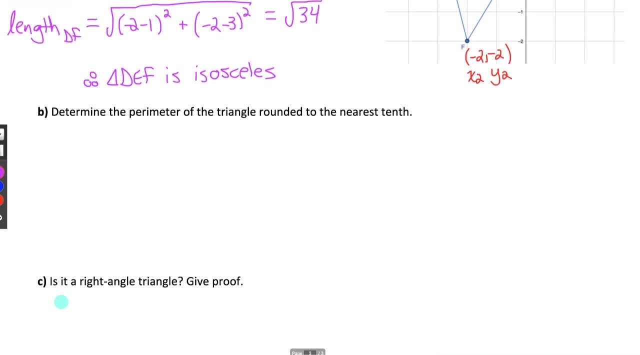 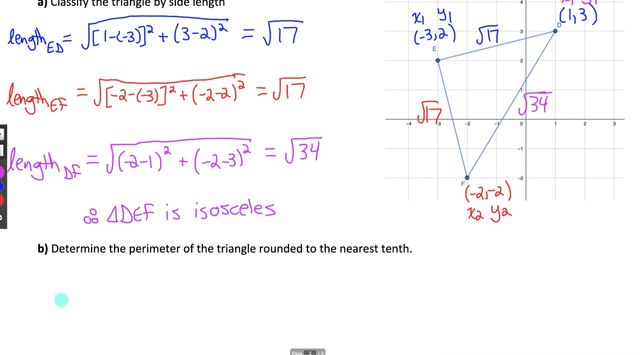 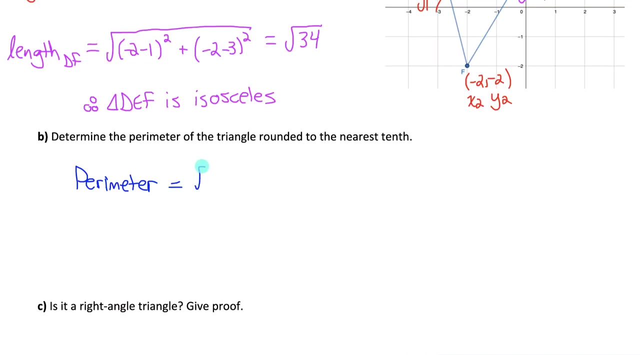 triangle. part b just asks us for the perimeter of this triangle and it says to round it to the nearest tenth. so we just need an approximate perimeter. what about the perimeter of a triangle? I just have to add the length of the sides. The perimeter would be equal to root 17. 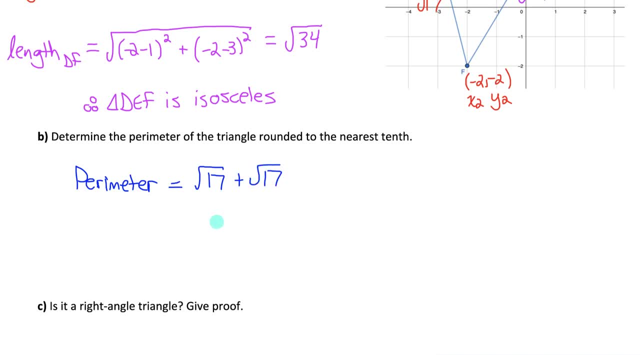 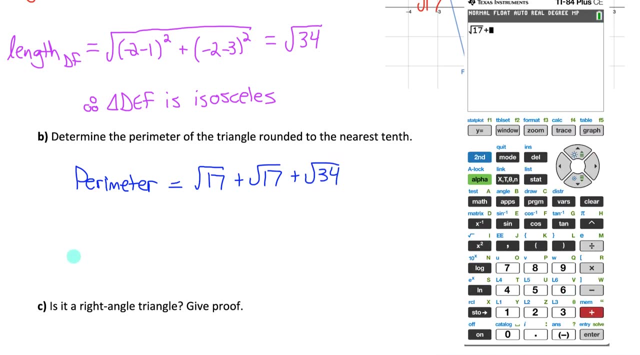 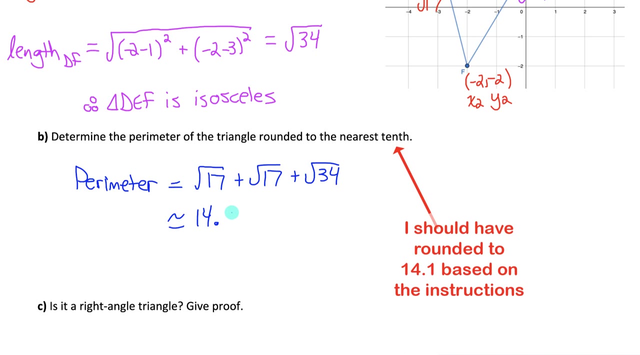 plus another root 17.. I suppose I could have written that as 2 root 17 plus root 34.. And it asked me for the approximate value, so I'll evaluate that on my calculator And that gives me a perimeter of about 14.08 units. Part C asks us: is it a right angle? 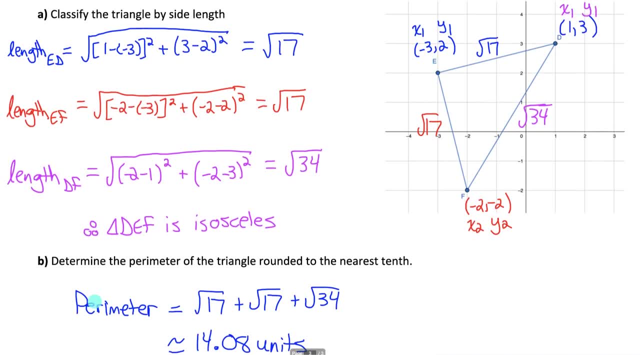 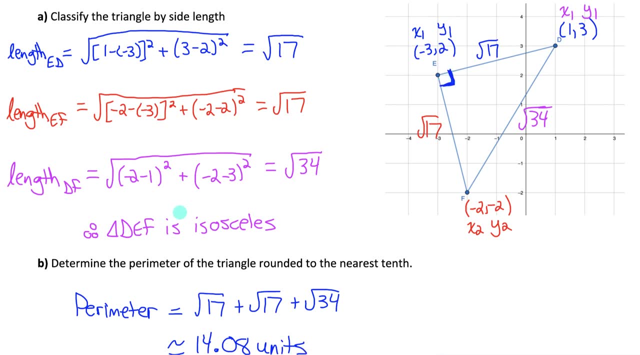 triangle Give proof. Well, if I look at the triangle, it kind of looks like this might be a right angle here. but we don't want to have to just guess and we actually don't have to calculate any angles. What we can just do is check if Pythagorean theorem holds true. We know that. 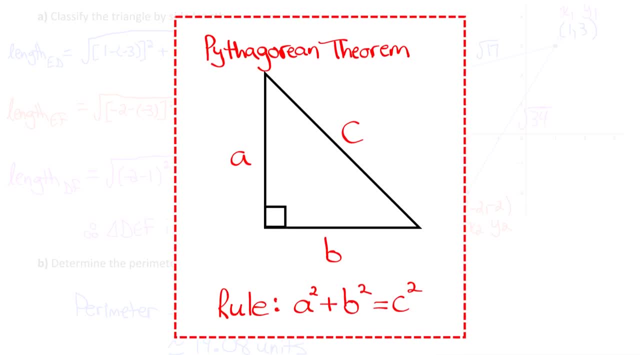 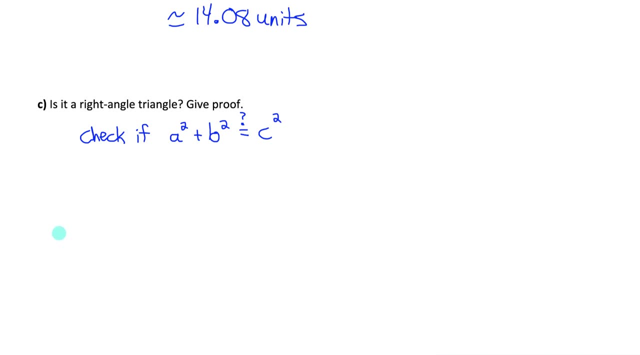 for all right angle triangles, the sum of the squares of the shorter two sides equals the square of the longer side. So let's check. I'll use the shorter two side lengths as a and b, So I would have root 17. Squared, Plus the other root 17 squared, And we're checking to see. is that equal to the? 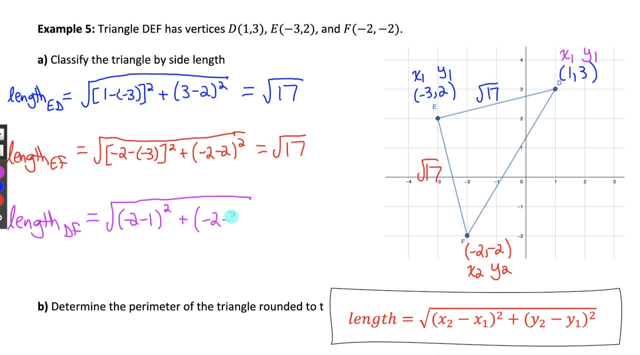 So this is negative 3 squared. Y2 minus y1 would be negative 2 minus 3 squared. Simplifying underneath the square root, the difference in the x's is negative 3, the difference in the y's is negative 5.. Negative 3 squared plus negative 5 squared is 34.. So this would 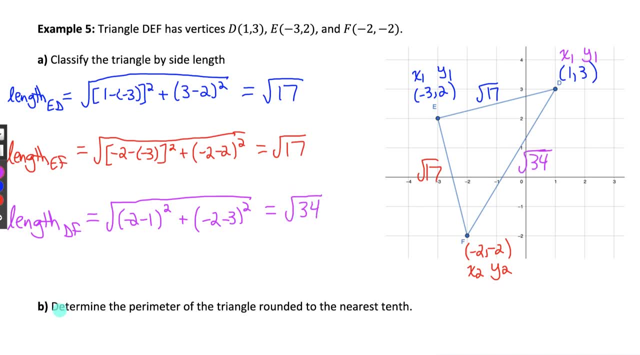 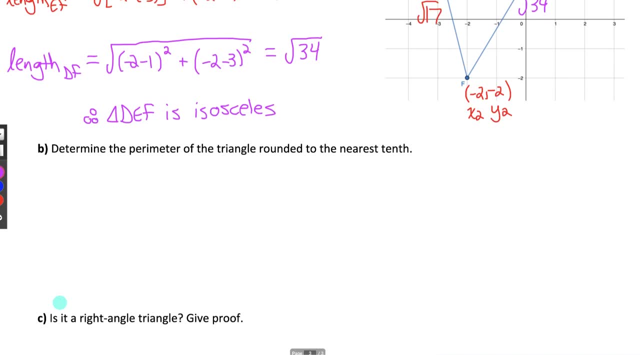 be the square root of 34.. Now that I know that two sides of this triangle are equal, I can classify this as an isosceles triangle. Part B just asks us for the perimeter of this triangle And it says to round it to the nearest tenth. So we just need an approximate perimeter. 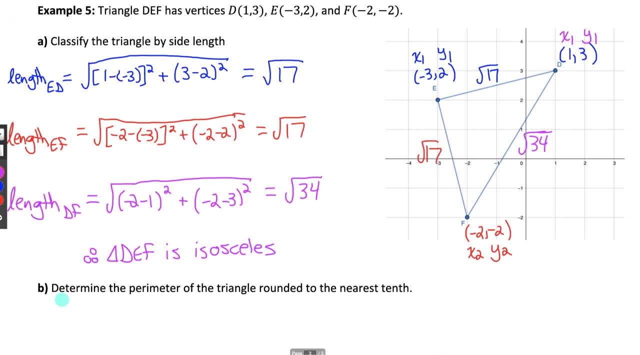 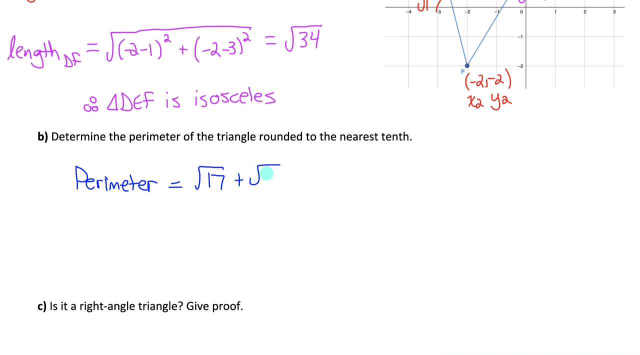 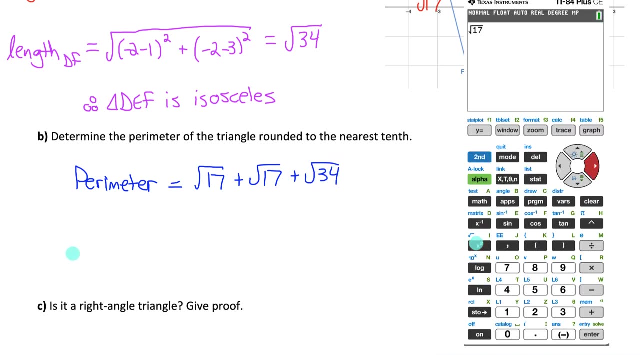 If I want the perimeter of a triangle, I just have to add the length of the sides. The perimeter would be equal to root 17 plus another root 17.. I suppose I could have written that as 2 root 17 plus root 34.. And it asks me for the approximate value. So I'll evaluate that on my calculator. 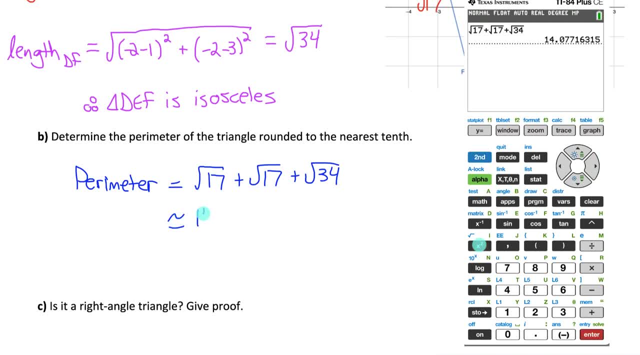 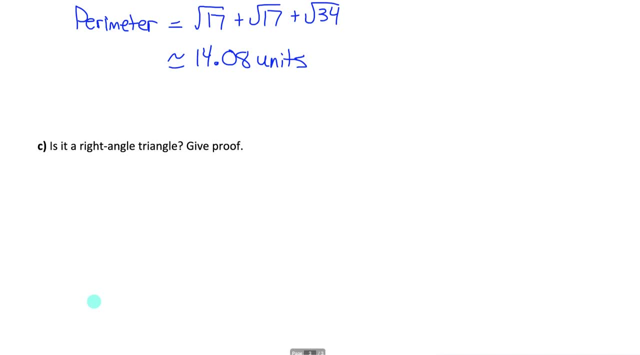 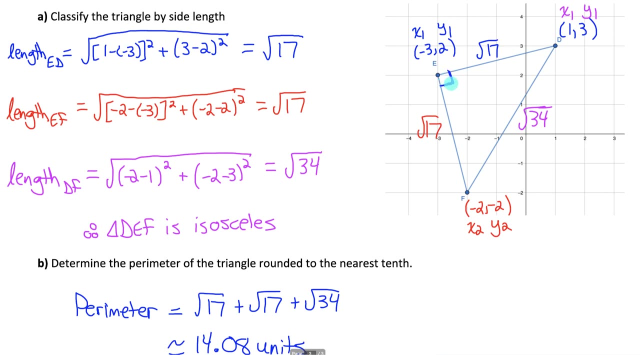 And that gives me a perimeter of about 14.08.. Part C asks us: is it a right angle triangle? Give proof. Well, if I look at the triangle, it kind of looks like this might be a right angle here, But we don't want to have to just. 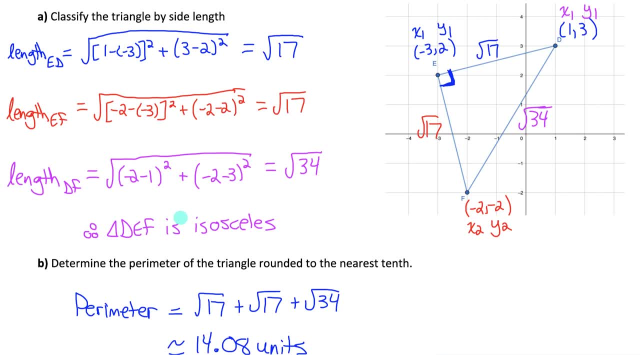 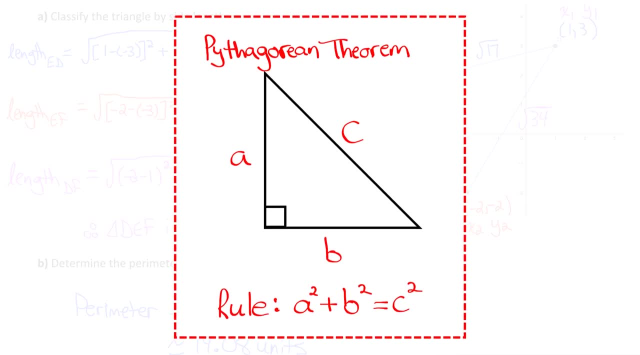 guess, And we actually don't have to calculate any angles. What we can just do is check. if Pythagorean theorem holds true, We know that for all right angle triangles, the sum of the squares of the shorter two sides equals the square of the longer side. So let's check. 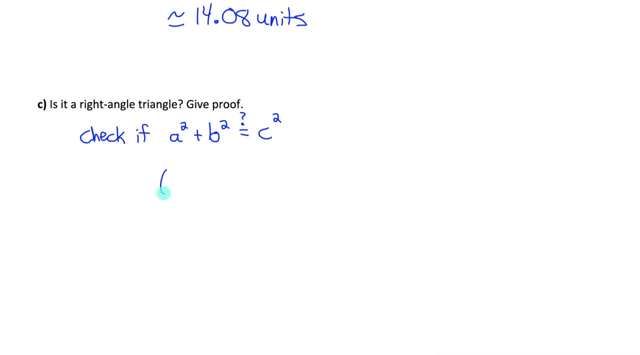 I'll use the shorter one And I'll use the shorter one And I'll use the shorter one. I'll use the shorter one And I'll use the shorter one And I'll use the shorter one. So I would have root 17 squared plus the other root 17 squared, And we're checking to see. 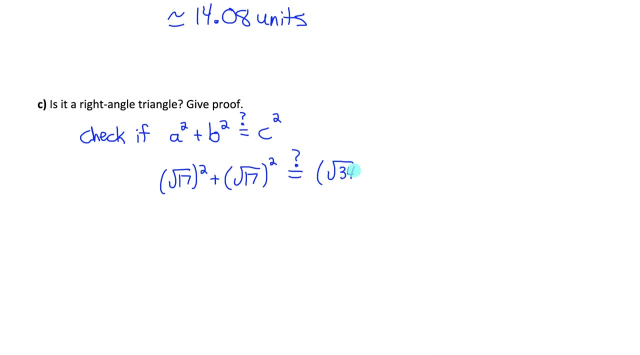 is that equal to the square of the longer side, which is root 34?? Is the left side of this equation equal to the right side? Well, hopefully you know that square rooting and squaring are inverse operations of each other, So they're just going to cancel out. So, for each of these terms, 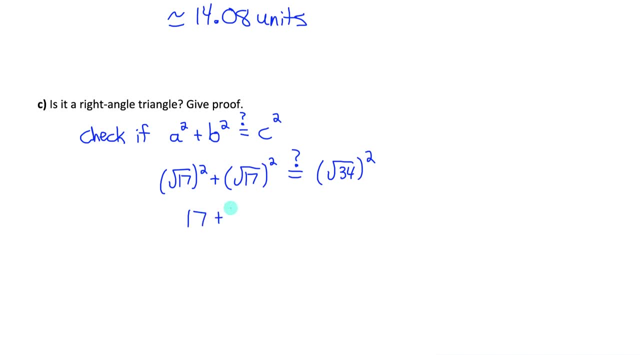 the square root and the square cancel out And I just on the left, have 17 plus 17. And on the right I have 34. And of course, 17 plus 17 is 34.. So the left and right side of this.